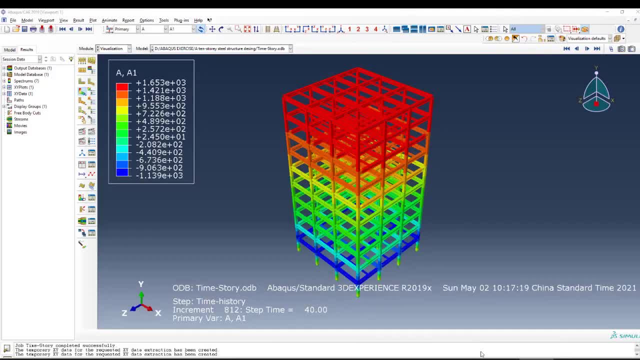 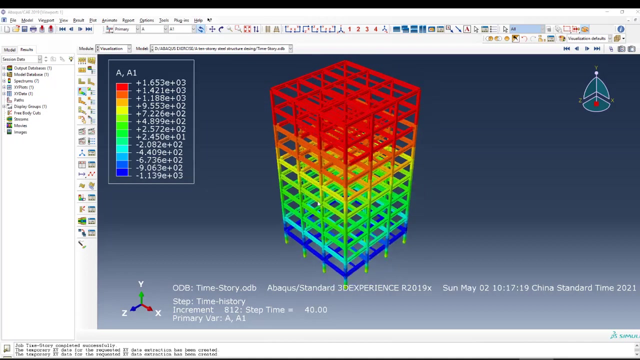 Hello everyone, In this video tutorial I'm going to show you how to model a high-rise building or semi-rise building or medium-high-rise building, steel structure or concrete structure in Abaqus software. After modeling, we will perform a time history analysis using a specific record from the earthquake ground motions. 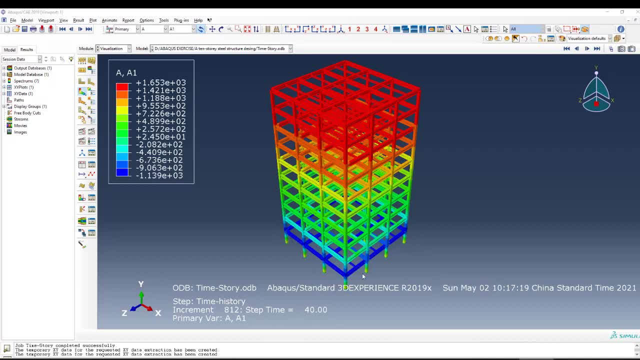 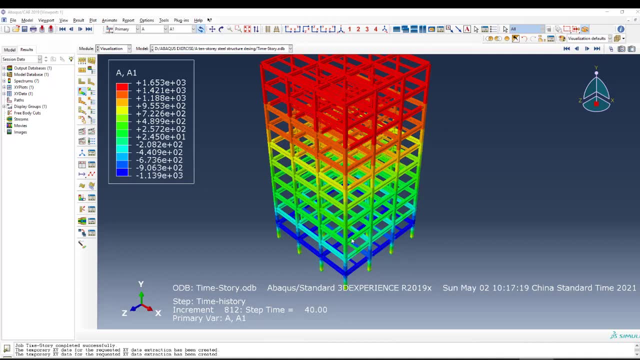 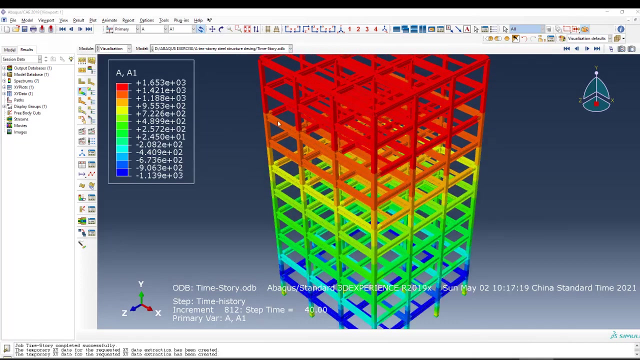 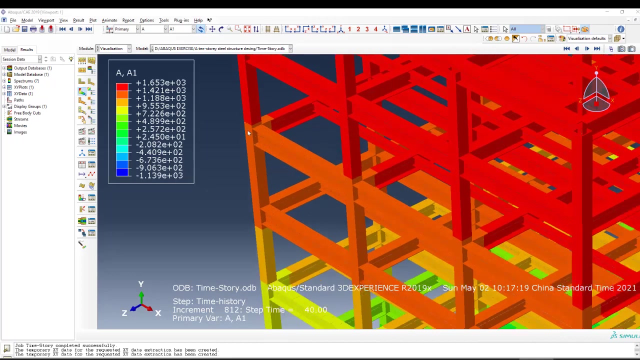 So for this case we have a typical steel structure which has three bays in X direction and three in the Z direction and about 10 stories in Y. Each bay has five meters and the height is three meters. So we use the two type of profile, three type of profile. One is for primary beams and the second for secondary beams. 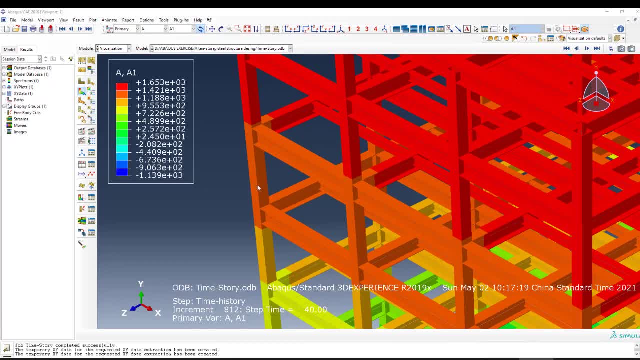 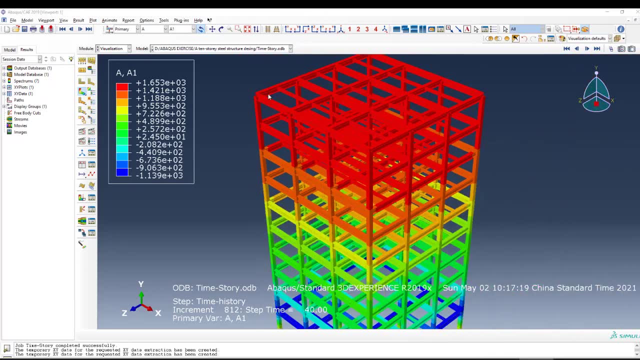 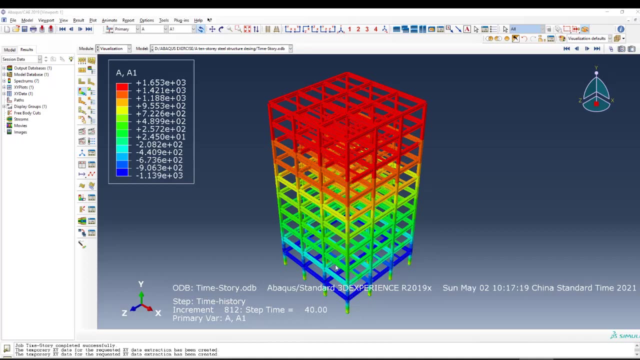 And we have a column. The column is from the box sections and the beam is from I section with secondary beam. So this is a part of result, That's the acceleration in Direction X, If we can assume that X is the north and C is east. so either we can apply in the both these two direction. 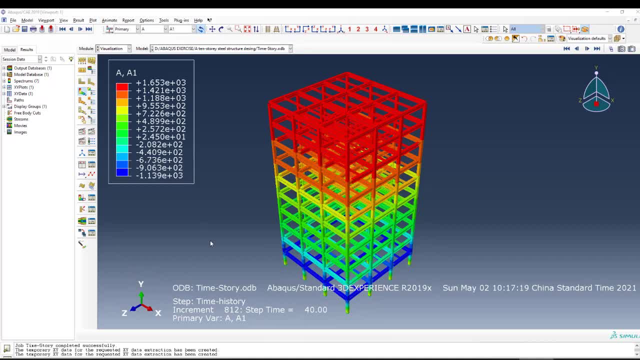 Even we can consider the vertical acceleration. So this is the result which, after analysis completed, we can see: the maximum acceleration is in the top of the stories. We apply In the ground, in the bottom of the structure, but the acceleration is in the top of the roof. 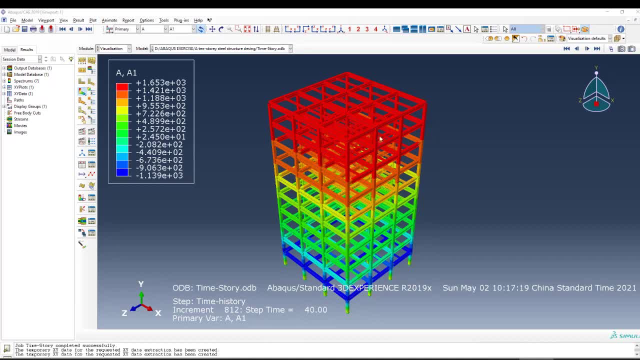 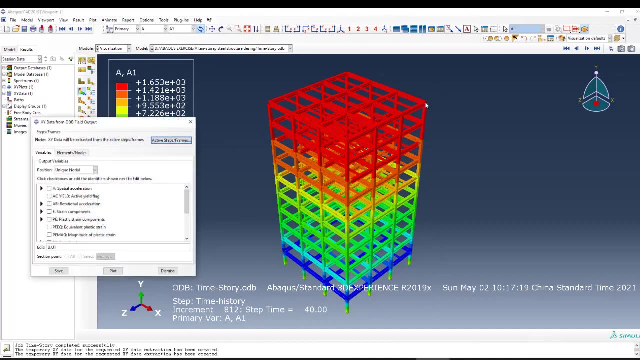 So this is the exact concept of the ground motion behavior. We can quickly check the output from the top of the roof and see what's the maximum acceleration in this roof. So here we can select unique Nodal and from acceleration we can get direct one and select a node. 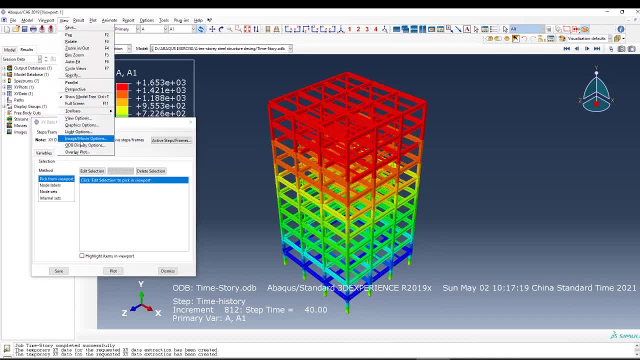 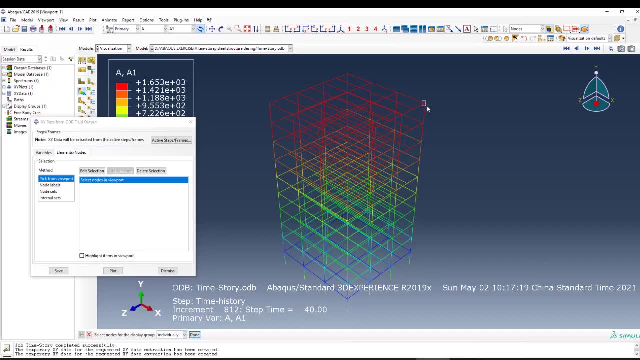 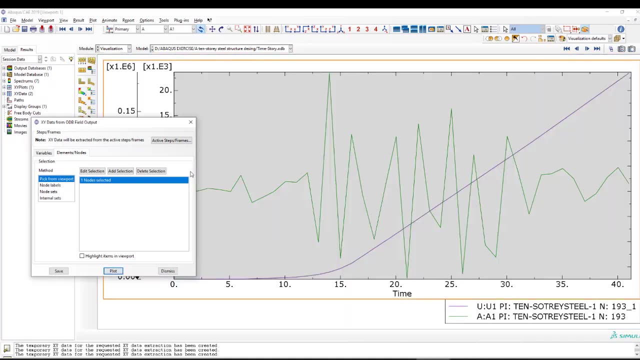 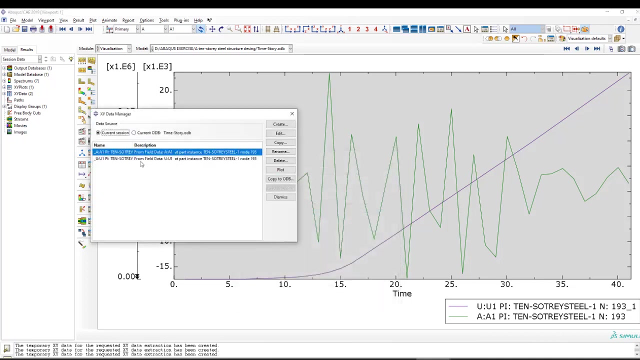 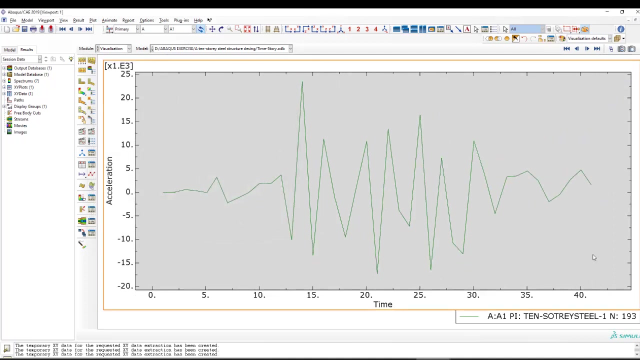 It's a rendering part. I'm going to off the rendering from here and we can select this node. So just this node is enough. and here is selected, We can plot. So this is the plot of This is the acceleration plot. The total time span is about 30 seconds. 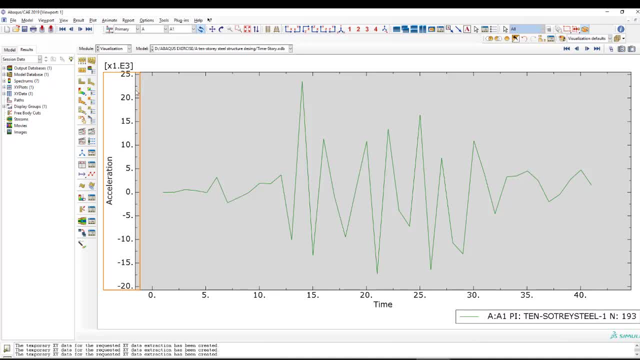 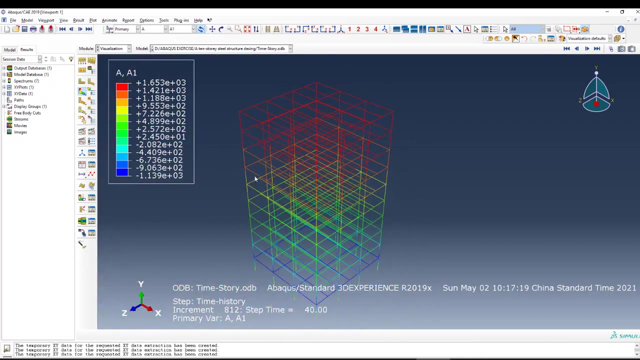 So, which is a maximum 2000, 20,000 millimeters per square second. So this is the possible result, And then we can see the deformation, deformation And also the velocities and other parameters. So OK, we quickly go to the model. 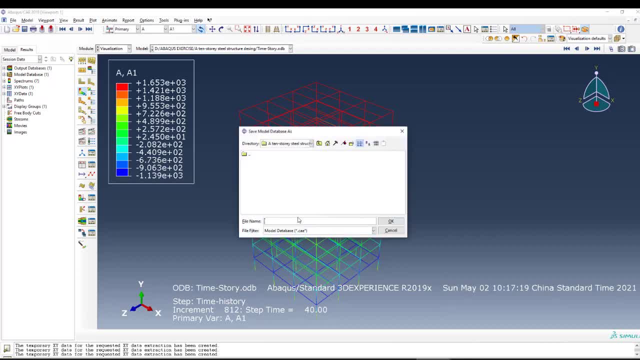 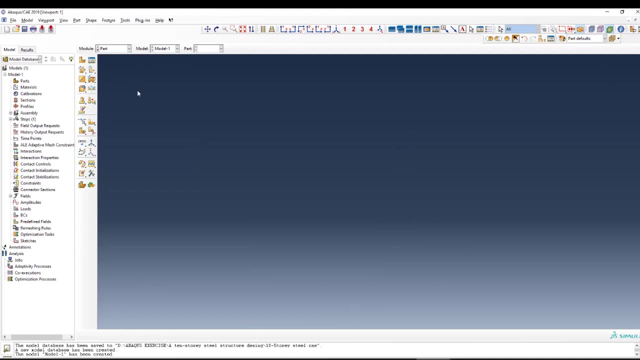 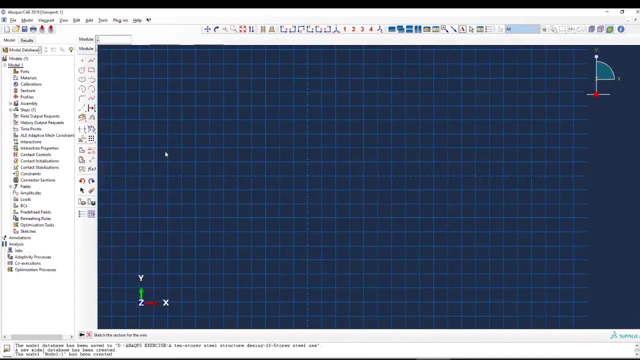 This, this one. I'm going to take a new one save. I save this one and I'm going to quickly draw another one, And this is the first I draw, called P beams or primary beams, is using a wire planer and using millimeters unit. 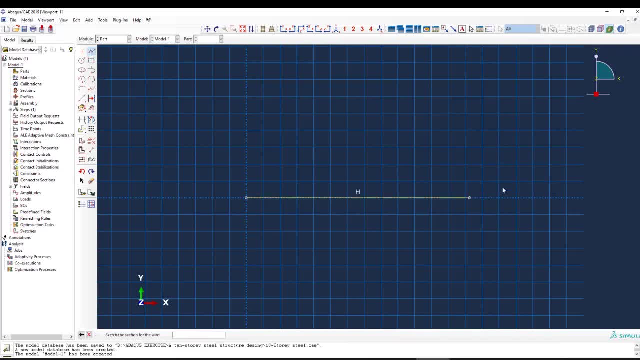 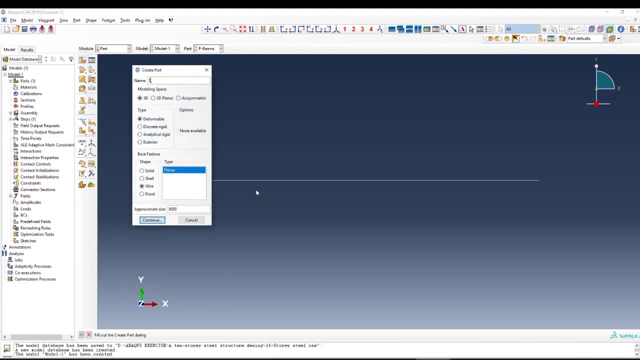 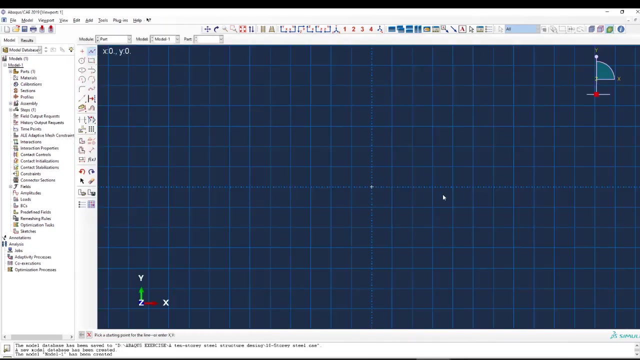 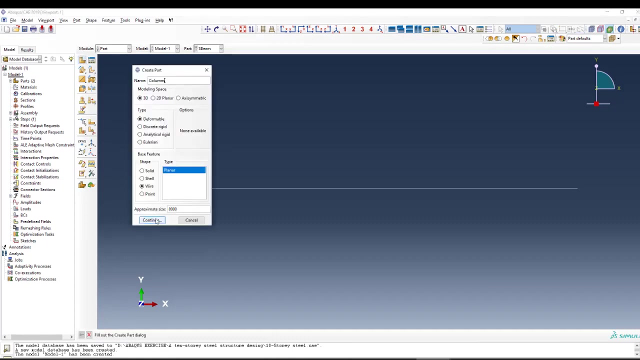 So the beam length is about five meters and I can quickly dimension Five meters, 5000 millimeters, and this is beam is done, going to call the ace beams, which is secondary beams. so the length is the same: five meters, five meters and the next drawing columns, the second is the third one is going to draw columns, the 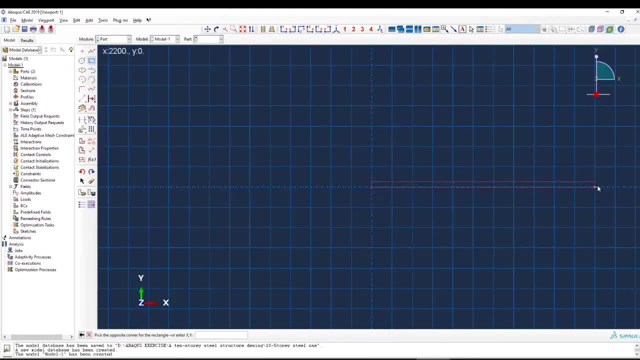 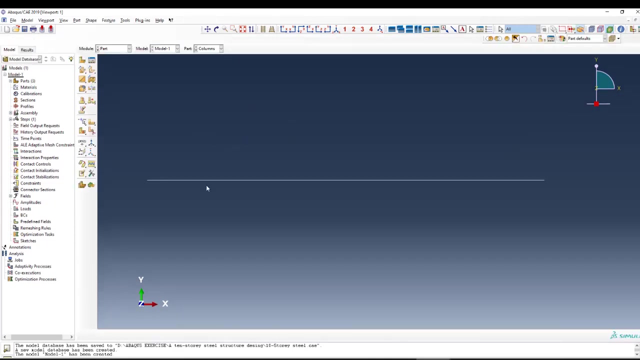 column ID is. it can be different. I want to draw a column which is three meters, very typical three meters, and this is done so that three- secondary beam, primary beam and columns or model, and next we're going to the property, define a concrete properties. so I have already saved. 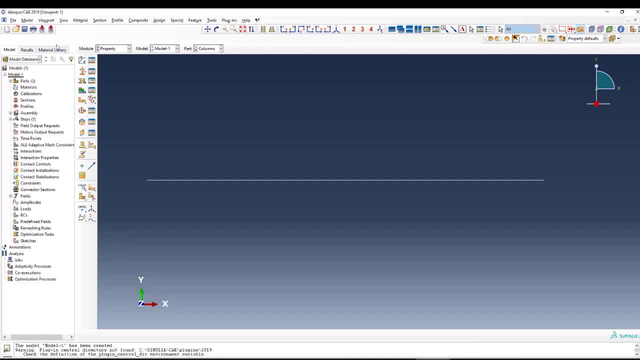 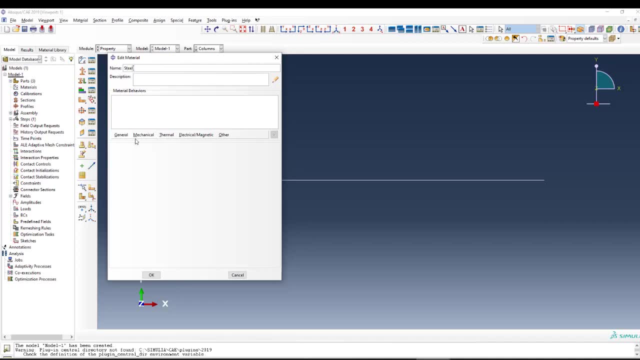 some materials in my library and I'm going to show you how to save a material. let's see, I called steel steel and here is giving the properties. just give elastic. this is elastic. and I'm going to give 200, 200 thousand mega Pascal for modulus velocity and 0.3 portion ratio. so this is a yeah. 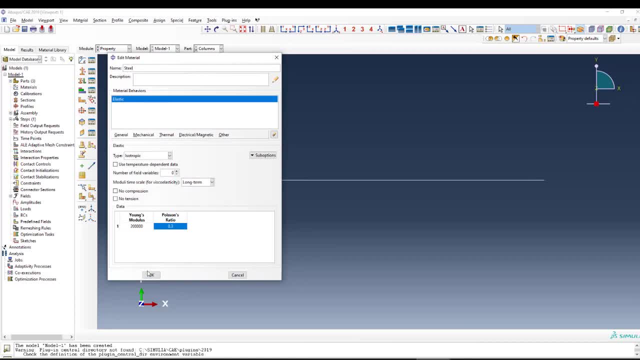 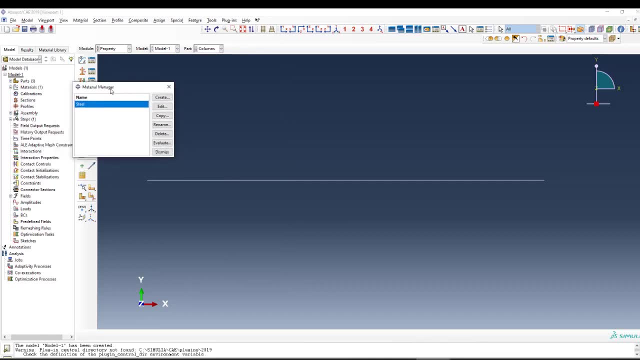 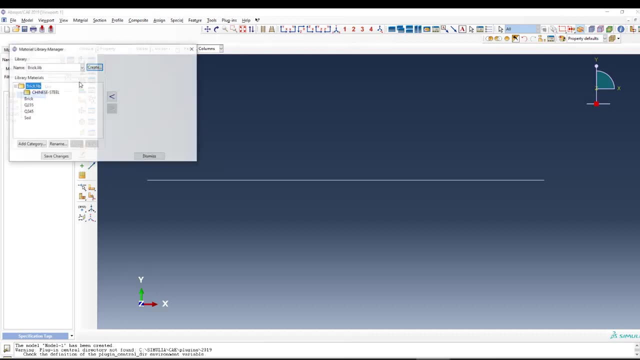 here should be something called steel. we have a space still now. we have a steel material, but this is elastic. I'm going to save to my library into the save to my library here now clicked here, click and we have a steel in in my material. so I'm 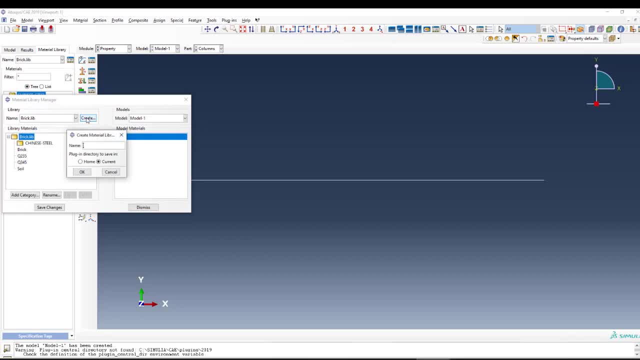 going to. I can select any. call the elastic elastic steel. so under this folder I will, uh, under this folder I'm going to add this steel. so now, yeah, save, so I can delete this and that. that. let's see, we have next time and came so that here and from here we can find that elastic. here is here. 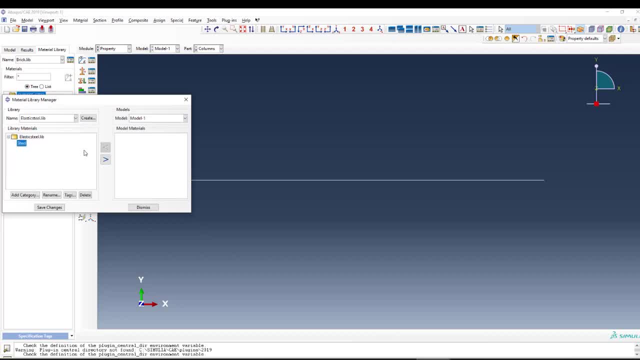 elastic, elastic steel and when you open here is still so. now we can add it with less distance. just add with less distance, and it will come back again. so we don't want to use this steel and I have another. I have another steel material that's using low schools from curve, which is drone. yeah, complete this isas and this is. 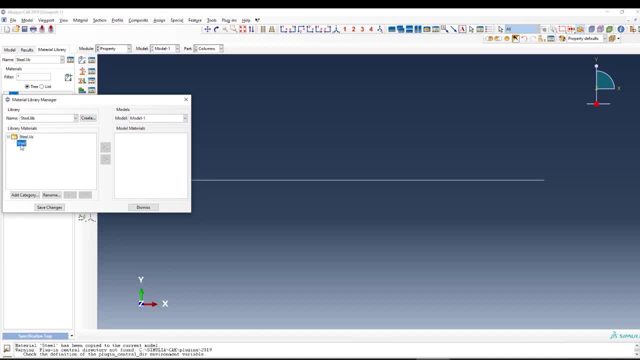 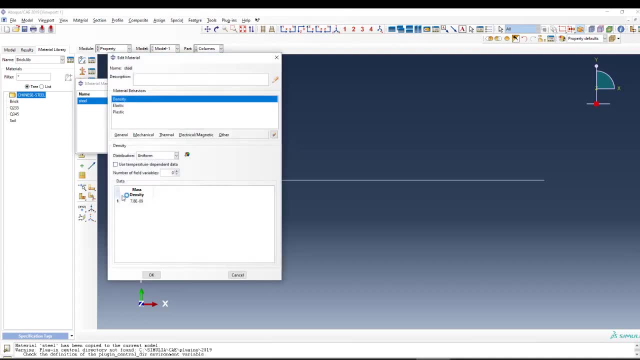 uh, actually we got from experiment, so I- uh, this is still, I'm going to still. now we can see the parameters we have is the first density, and the second is elastic and the last one is plasticity. so i have drawn this curve and the maximum ultimate is 400. 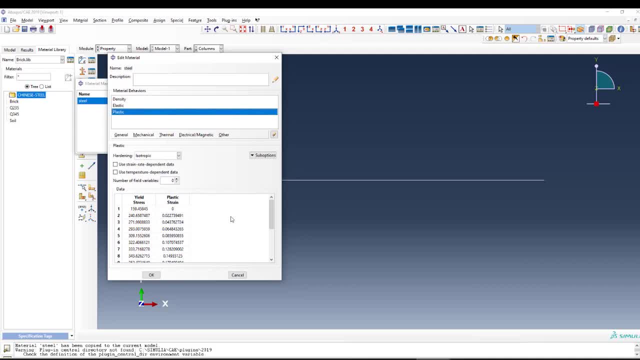 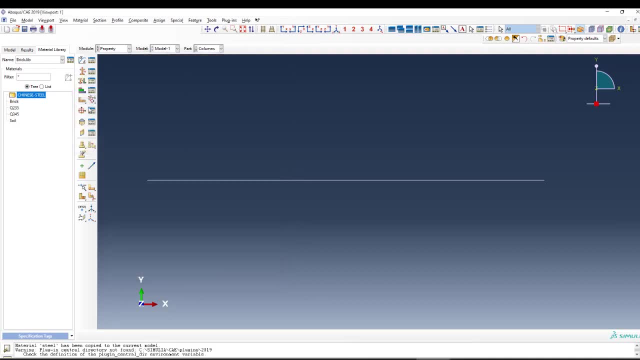 and it's uh still s certified, which is using uh russian steel codes. uh, okay, the next is, we want to draw uh three type of profile. one is for primary columns, uh, for columns, let's see columns. this is a box section. for box section, this is a square section we have. 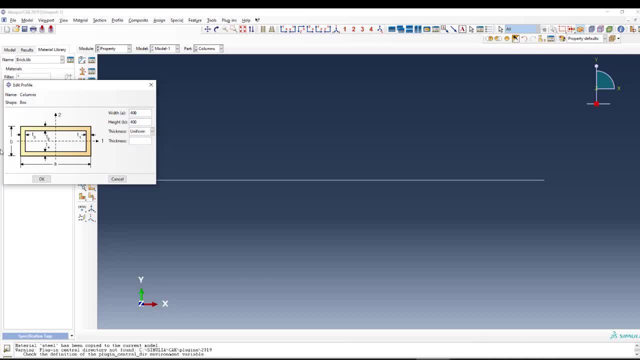 400 by 400 and this uniform thickness in across this section is about 20 millimeters and the next profile is uh p beam which is a primary beam and using i section, so the total uh- the midpoint of this uh section is a 250 uh. at 250 uh we want to use the 500 height. 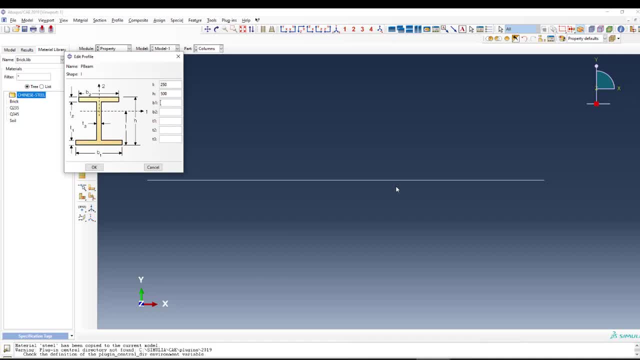 and because it's. we have some primary question equation that's called l divided by 8 to 12, so we can take the average and we we can select the height of the beam for primary design. we can see the response of the structure and after that we can optimize which height is quite good. so the length is should be 400. 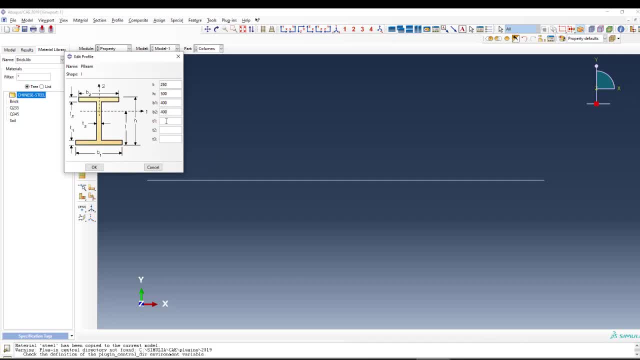 which is similar with column and 400 and the thickness one. thickness two is flange, so we can use uh of 15 and also 15 and the waves can be 10.. this is the primary beam. we have a secondary beam called s beam and the s beam is the maximum is 130 for main point and it can be 300. 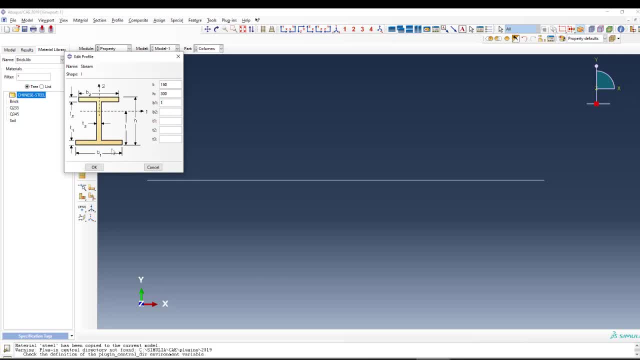 so this is also 100, uh using 150, or you can use 200, 200 flanges and the thickness of flange is about 10 millimeters, 10 millimeters and it's 8 millimeters. this is done. the next thing is: uh, we're going to pop define some consection c equal uh columns. 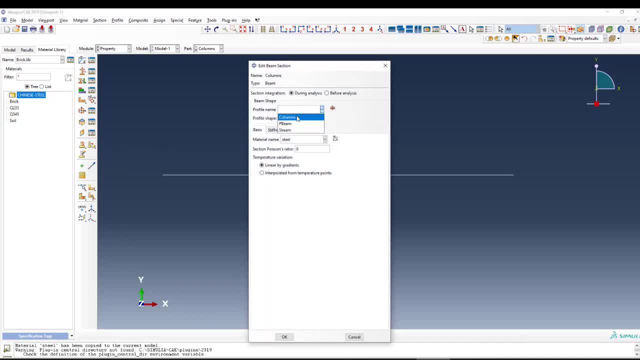 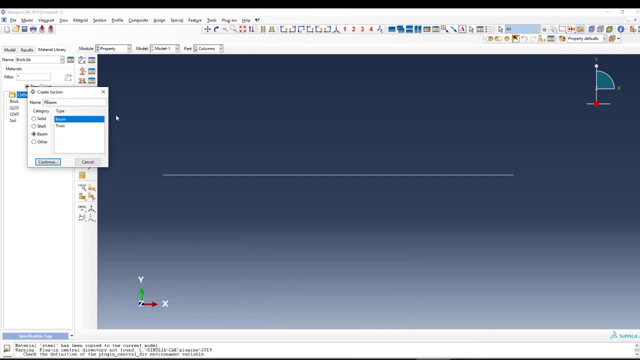 this is beaming elements and we're going to define some length to select the previous uh defining profile. so this is column and here is called poison ratio. we can give it and again, and next going to called p beams, p beams and here is select p beams. 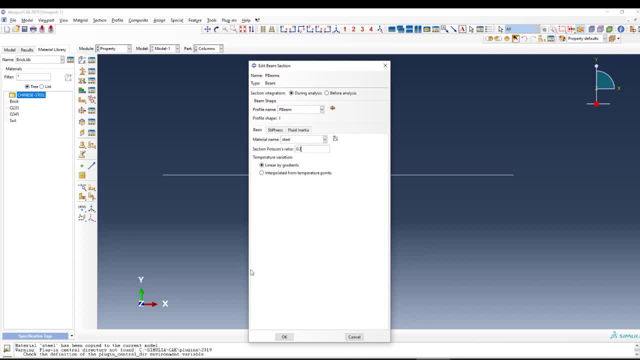 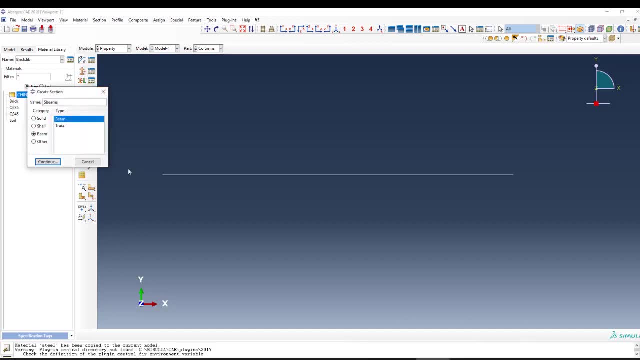 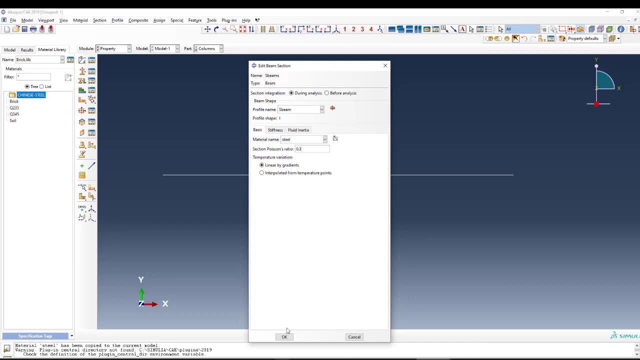 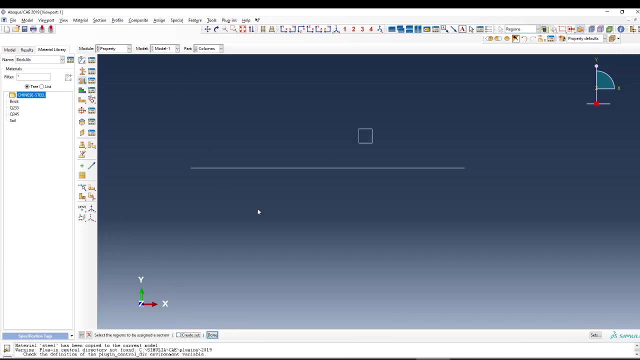 and the same materials, 0.3, and one more that's called secondary beams. the secondary beams selecting from the profile, and here is 0.3. so the uh, the section is defined, and now we are going to assign. so here is column, and i should select columns, columns, and next, 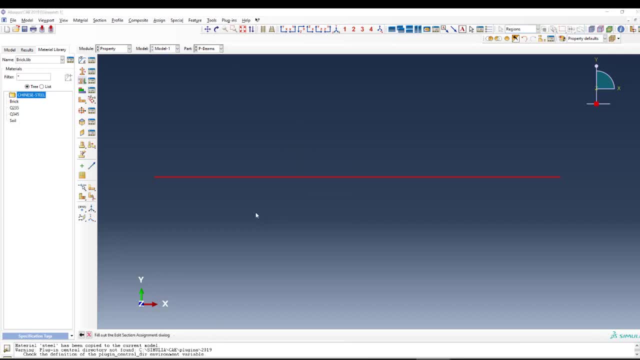 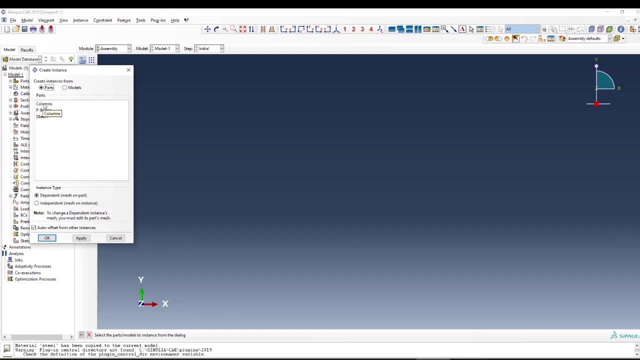 is a primary beam and i'm going to select: primary beams, p beams, and the last one is a secondary beams, secondary beams. this is secondary beams. okay, it's finished. and the next: uh, here we are going to the assembly. uh, we are going to assembly, and first, primary and column should be add. 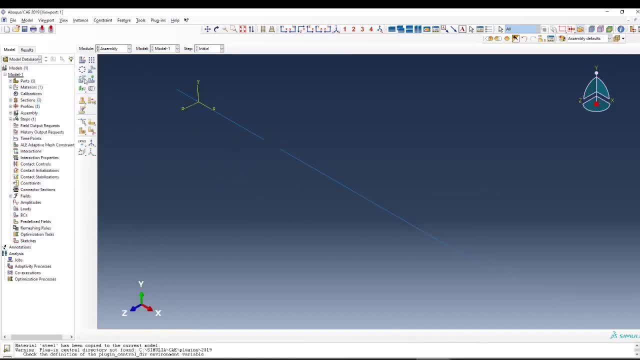 to that, here and now we are going to rotate this one and rotate this one, taking this point, and it's 90 degree, let's see 180. no, we should select this one. uh, i'm going to rotate in this direction, good, and this is actually column, and i'm going to put this point to the center and next i'm going. 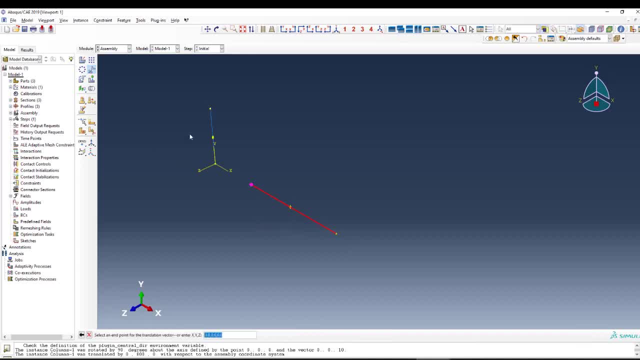 to select this one and here to this join. then i can use linear patterns and copy both of them in. this is 500, this one. and let's see direction: i can select this direction and for this direction i can use uh, this direction. so we are going to use like like this: uh, one bay, two bay, and this is a three bay. uh, it should be. 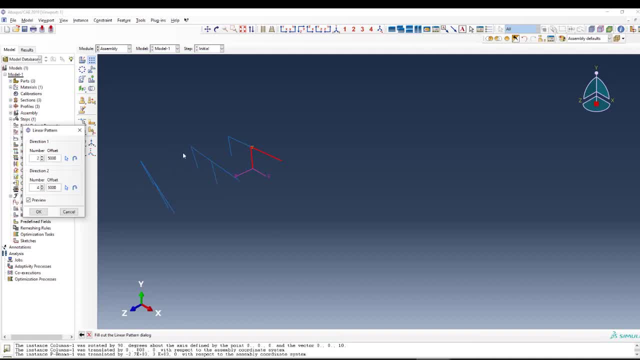 500, 500, 5000, the same like this, and here is uh going to front, uh, front, uh, this is uh one, two, and it's one, two, three, uh, okay, and the remaining part is here, and i'm going to quickly, uh, uh, quickly, i'm going to off this and 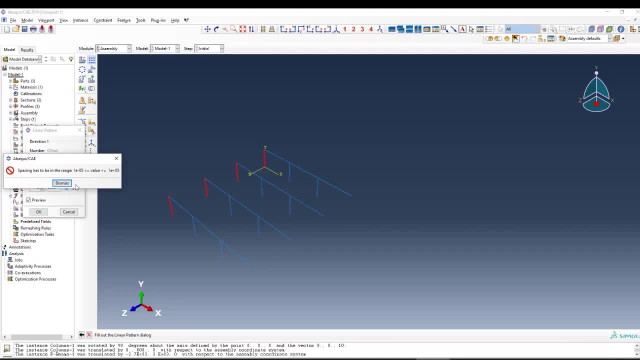 and here is going to back, and here is going to back. okay, and i'm going to select- sorry, should select this- this one here, and i can change this data to about 3000. yes, so don't need this one and i'm going to quickly, uh, uh, uh. 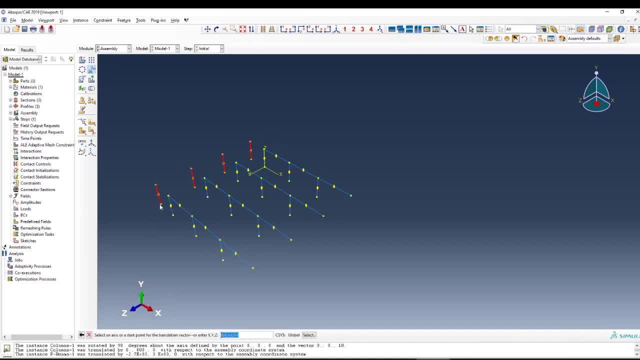 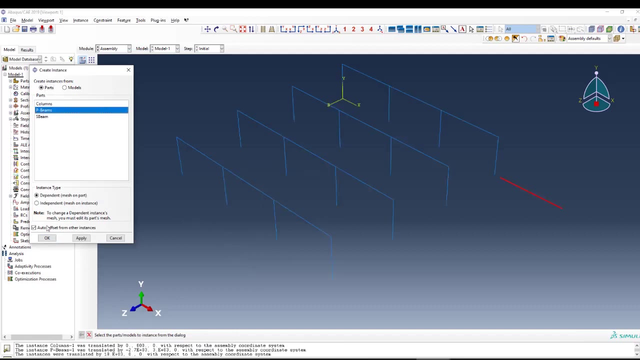 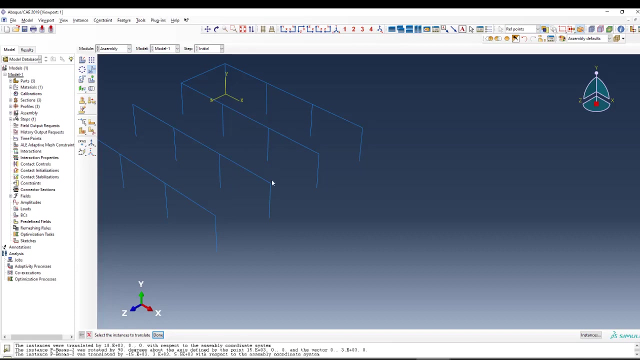 Select this one. You can select which way is better for you, And I'm going to bring these four columns here And next I'm going to input one of the beams- primary beams again to distribute in this direction, Z, And I should rotate this and take these two points and it will quickly rotate like this. So I'm going to select this one and select here to here, Now again using this linear patterns, and I'm going to give about 5000 in this direction. 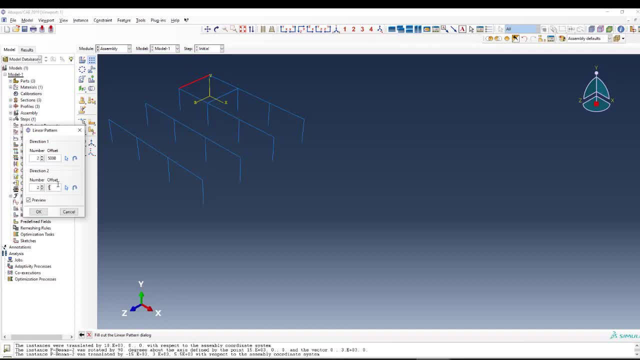 And here is also 5000. I'm going to select these two. So this region and this. Now, here is that and here is also that. So one bay two, bay three. This is quite good. And next is the same patterns. 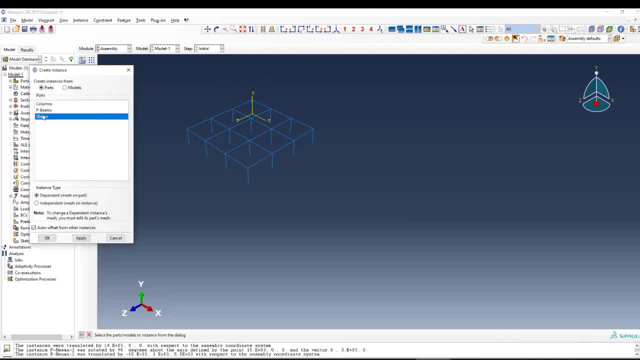 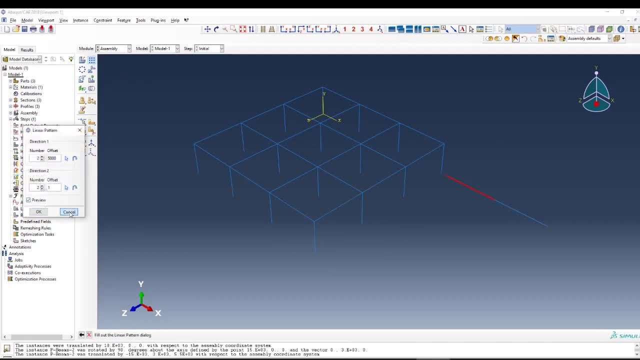 But wait, we have to provide that secondary beam, Secondary beam as well, Secondary beam. I can quickly take this secondary beam- Sorry, Move this point- and using one single secondary beam. So, and I'm going to select this secondary beam and I used 500 and I should select this direction is also 500. 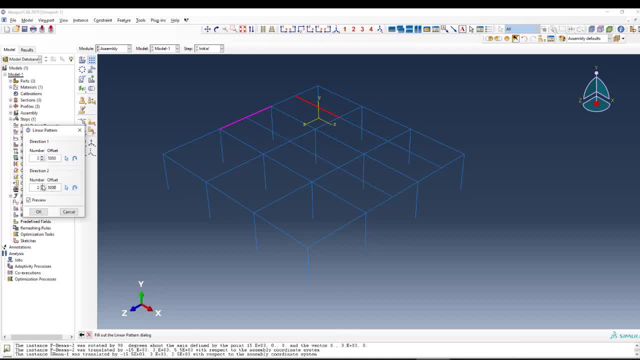 Using this one here. So this is enough And this is enough. Okay, Now the first floor is completed. Now select all And we're going to turn off this one and increasing this one is 3000.. We should use this app. 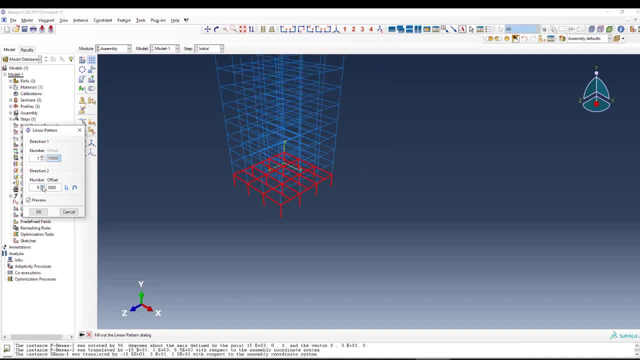 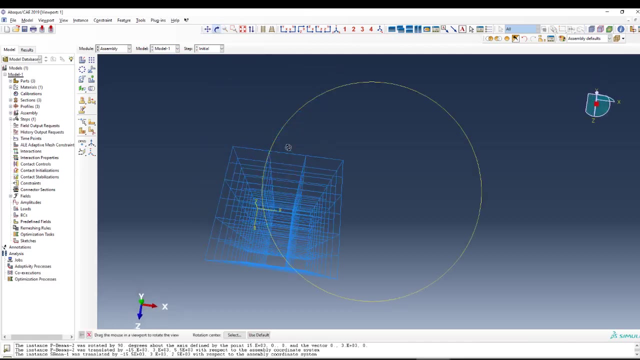 And now we can. it should be 10.. This is 10 stories: One, two, three, four, five, six, seven, eight, nine, One more, And this is 10.. So this 10 story is done. So we draw all the system Now. the next is I'm going to: instead of using some sort of connection, we used a fixed connection to each beam columns. 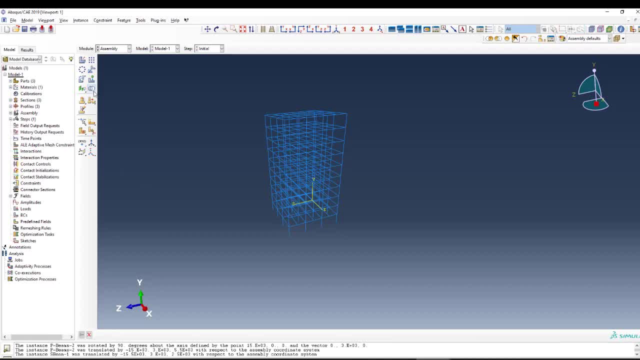 Okay, So all this, I can say 10 story still- structure the subways and you should call the retain and select all the system And it is done. Now it's become a single structure. So the next stage we are going to. 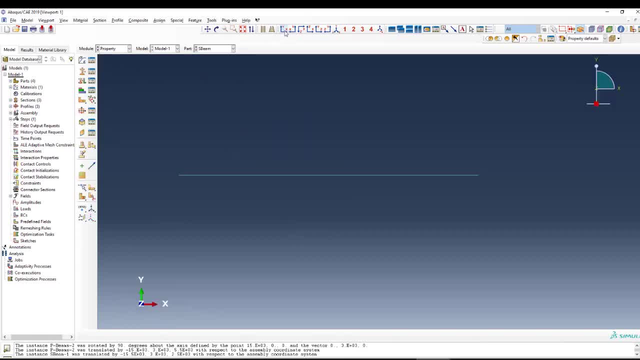 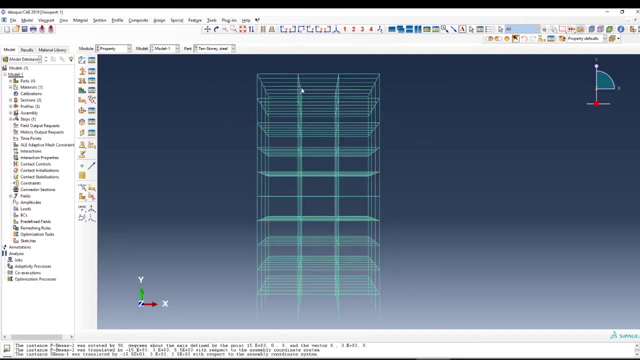 properties pack and we are going to apply the orientation so that orientation can. here is a section, The section should define orientation. This is the ocean to, this is one. So and I'm going to bring that 10 stories and here is X, Y, Z And I could select all columns first. 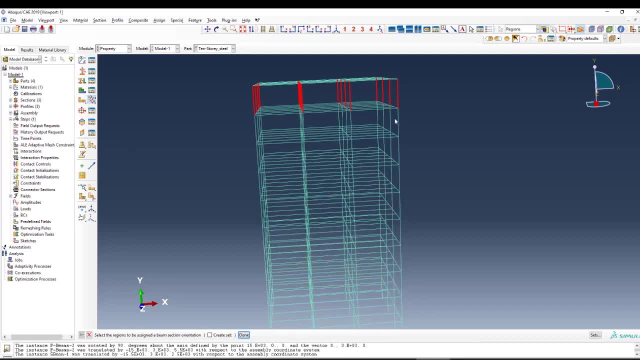 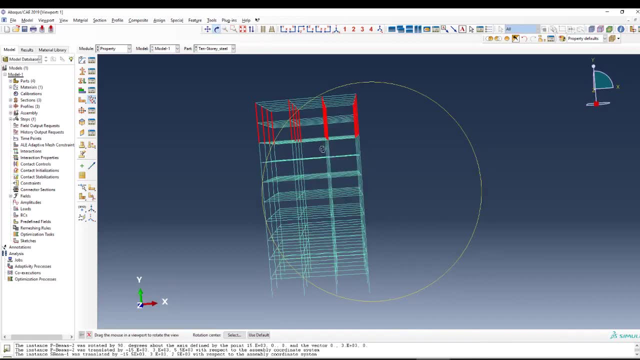 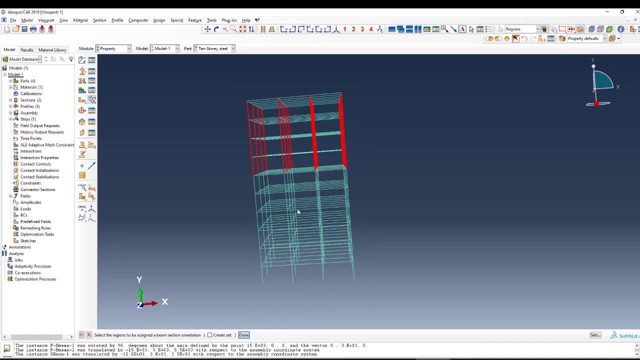 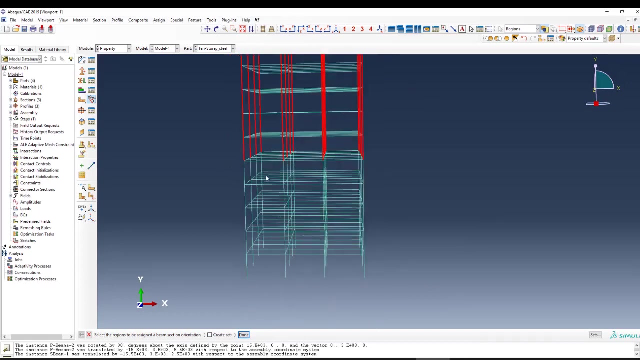 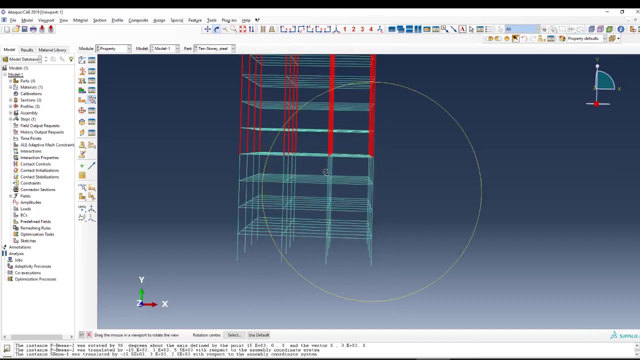 the column is a rectangle section, so it can be quite easy which direction you want. if it's two one, it doesn't matter. so both direction moments inertia will be same, but in the primary and secondary beam it's quite different. so I will show you how to handle this. 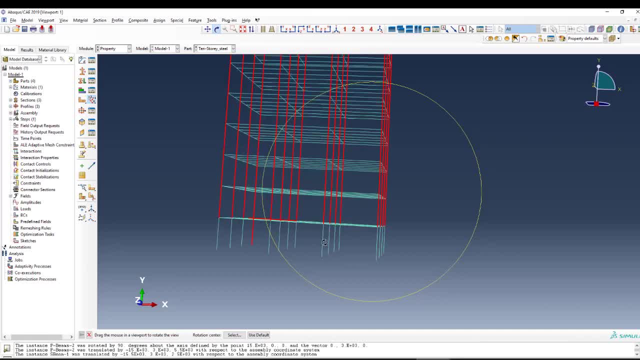 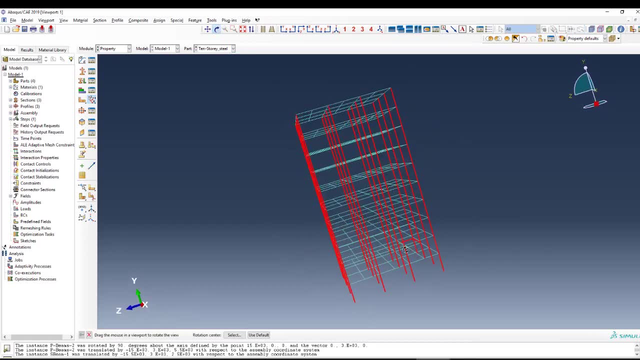 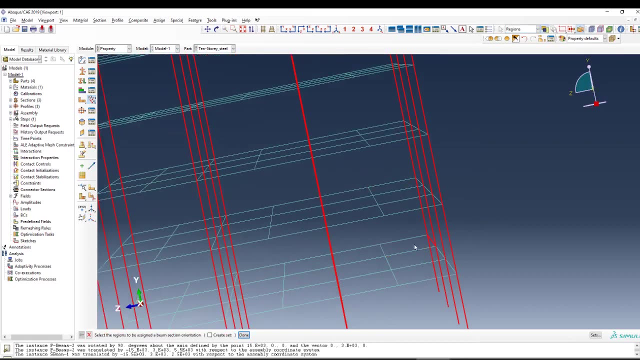 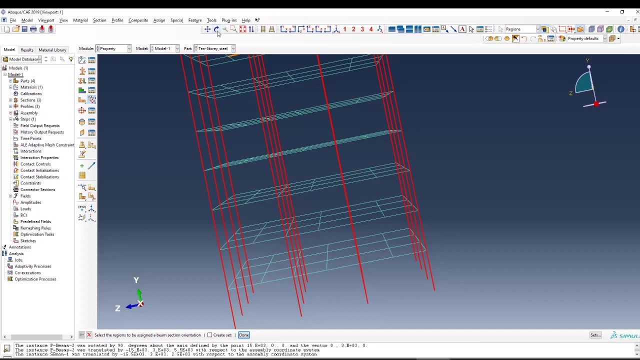 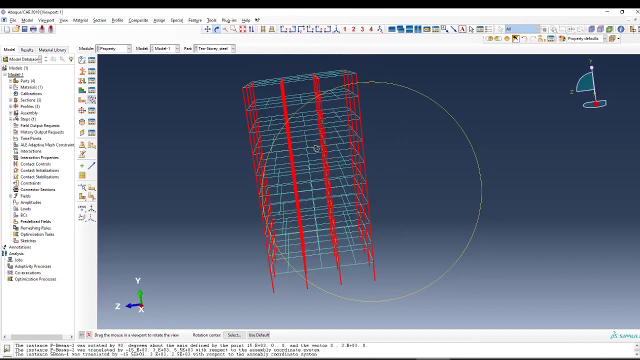 there is also some software. you can model this structure in ETABS sub and then then you can try to export to the input, the abacus software. but there is one, free, that doesn't work well, and other is paying, which is developed by dr chun. it's called dining chun and you can. 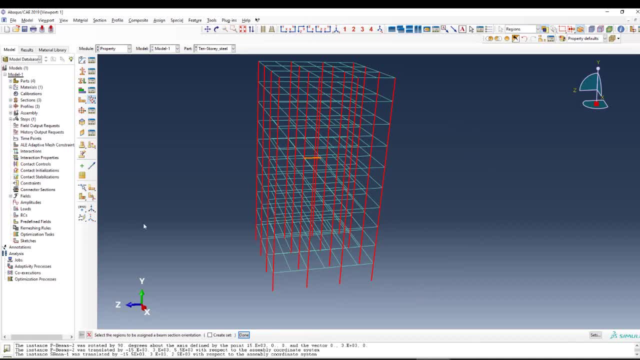 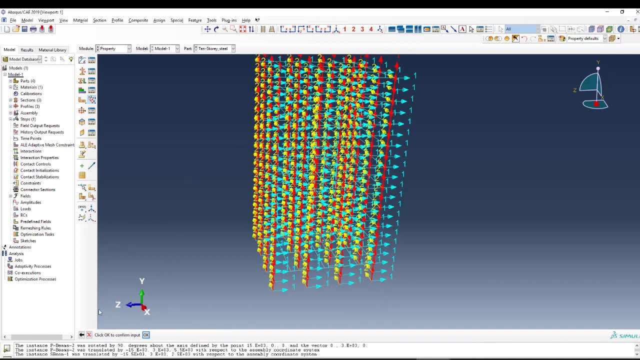 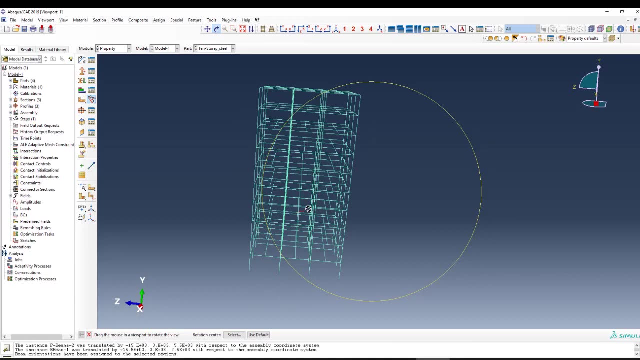 check his website and you can get that software called abacus, sub sub ETABS boss software. so now it's okay, I can give any of them is okay. so the orientation for column is completed. the next days we are going to show you how to apply for the beam. the beams, the same here, and I'm going to the eviction. this: 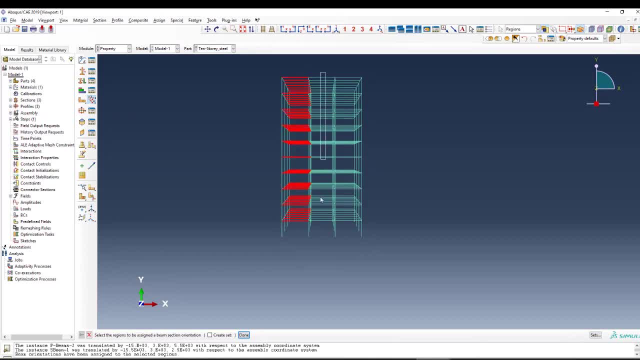 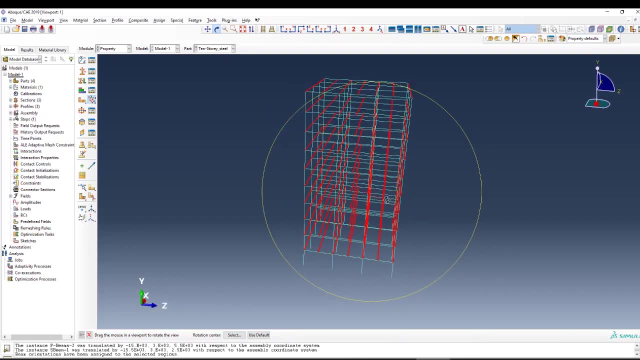 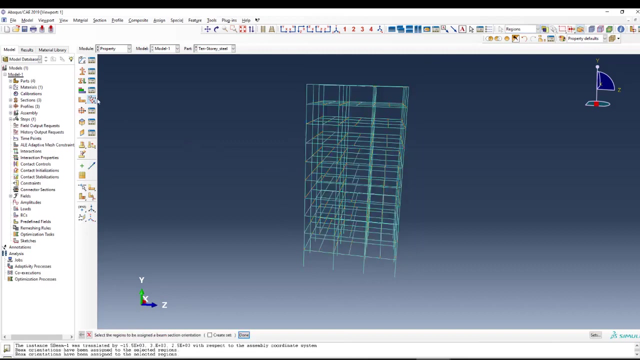 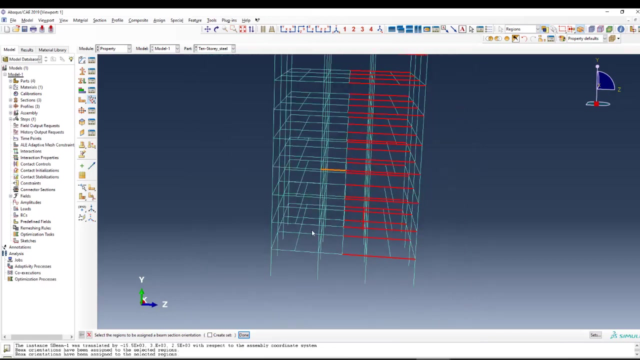 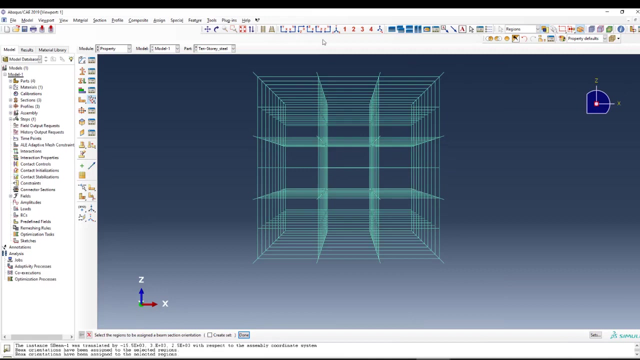 is one part and this is one part and this is all beam is. let's see here and we have selected all the beams and but other direction cannot accept these, we want to use other. okay, now again, again, these direction beams you I selected, maybe something I can again, I can, I hear it and I go to again select. 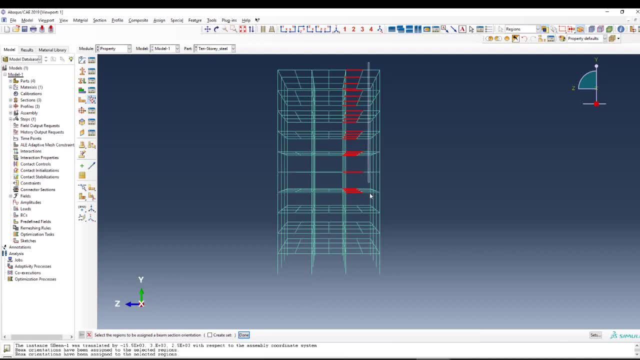 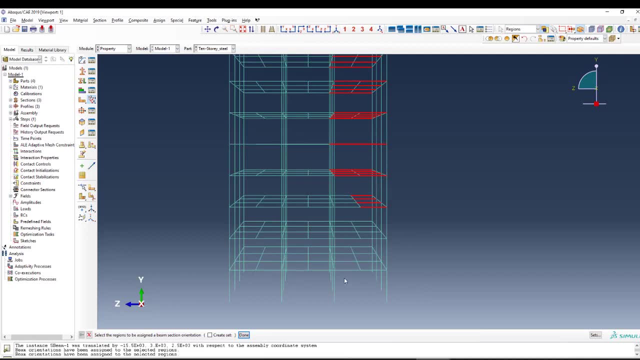 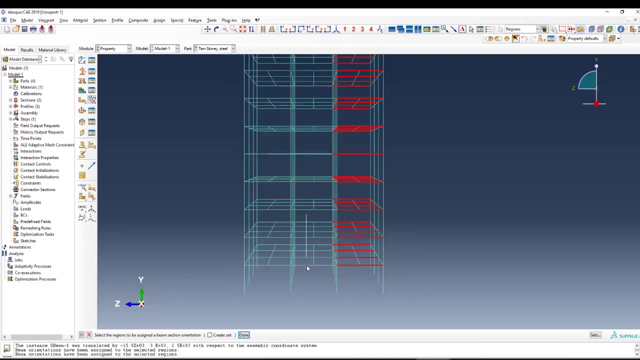 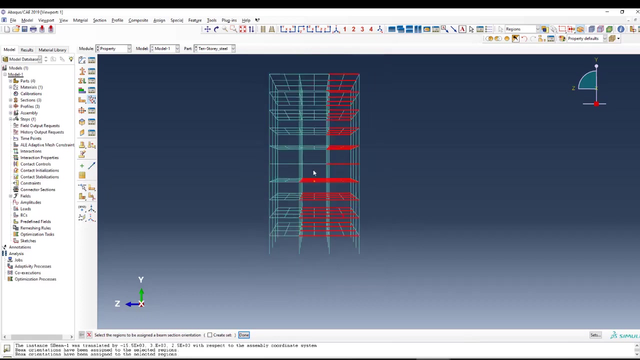 okay, and here selecting this and here. so all the beam is selected and I can give it a name. I can give that from the X one, so the number I can use zero and one zero. So this is okay, and now we can go to the assembly. 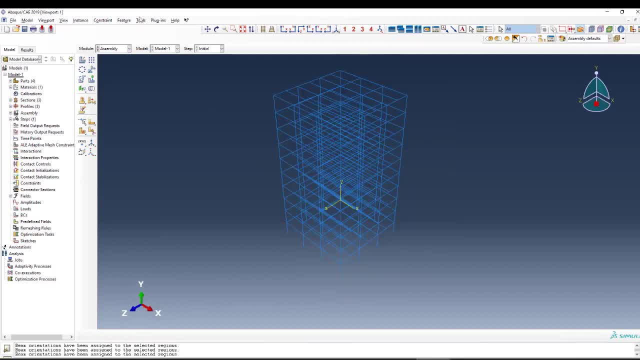 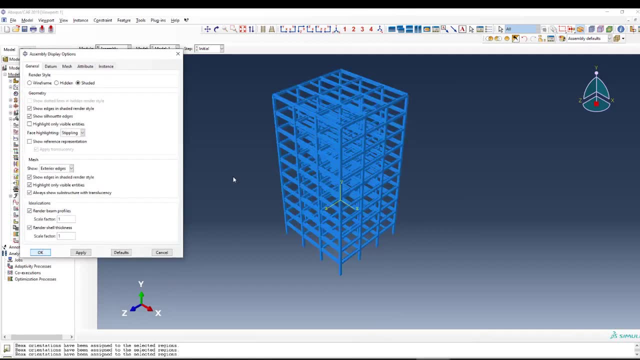 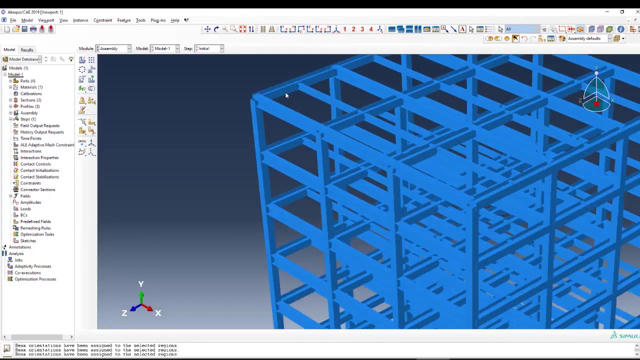 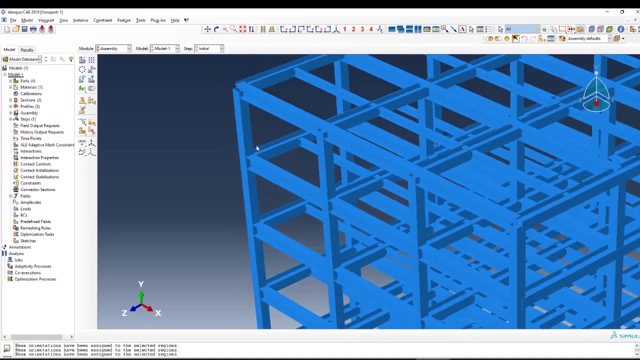 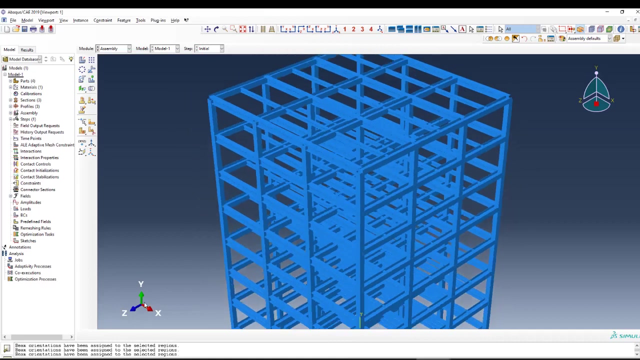 and check the front view assembly display and rendering beam and we can see which beam column is wrong. We can see this is right and but other one is wrong. So yeah, that second one. it shouldn't be in a Y. 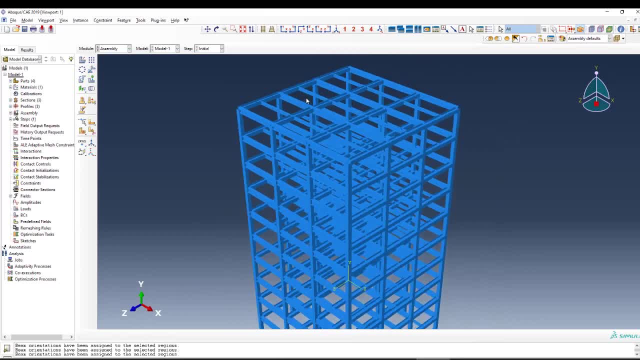 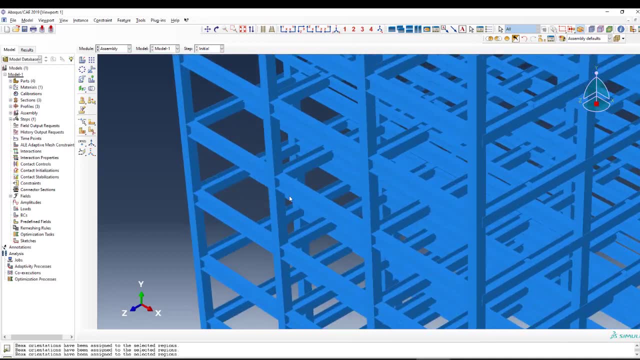 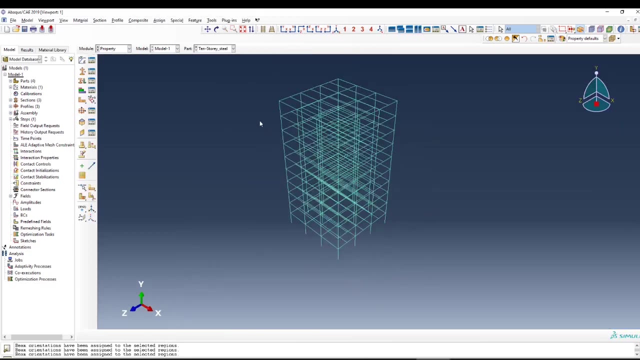 the number one should go to Y. so it's wrong. we can change, we should change it. So this is okay. and the next, this is check. the primary is also same. Only thing is that that here we should select again. 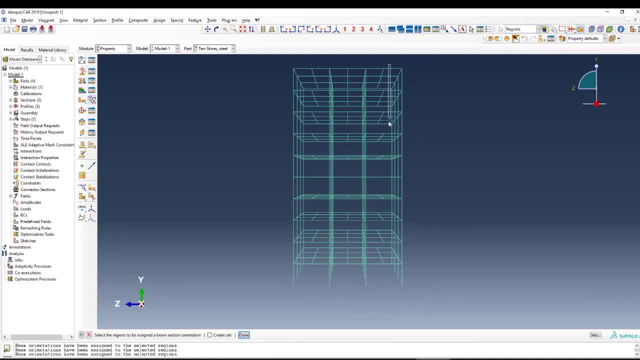 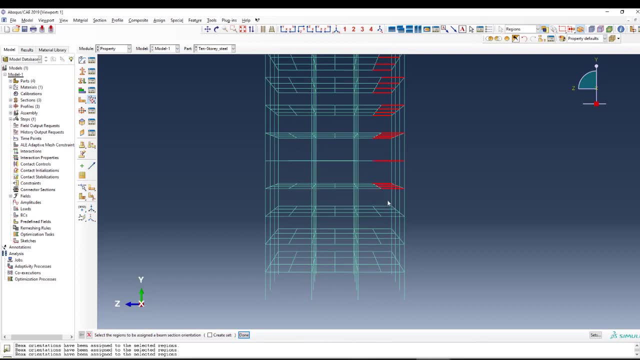 orientation and and I think that's good and I don't want to back up, so we won't do that And we can go back into, okay, and I've got a. there's something on the top of the screen here. 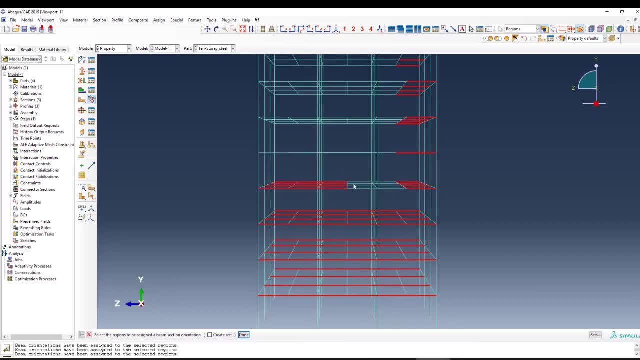 and we can just go through the top of the screen. So here's the bottom, this is the bottom. I say: take out the top, and then we put this back on and we can go back into our base. and now I'm going to say: 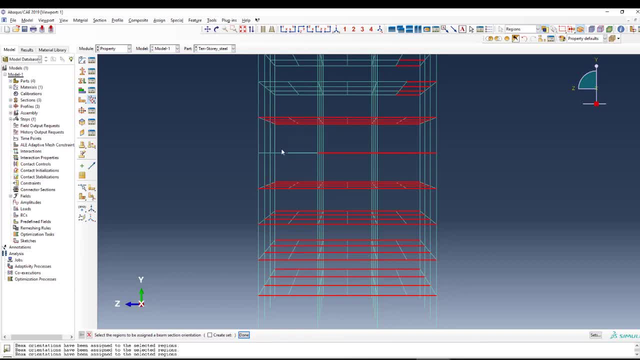 and I'll leave it like this. So I'm going to go over, I'm going to go over the top. I'm going to say: and I'm going to set up the limit. and then I'm going to say: and I'm going to say: 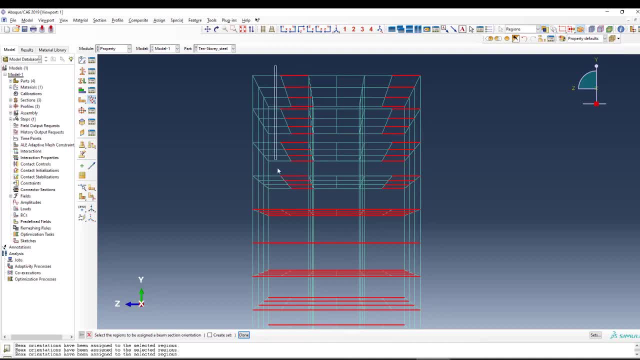 and then it's going to say: and now I should use a should be number one. so I'm going to use: yeah, this is okay, now we can go to back to the assembly and this time we can see it's correct. so this beam is in a right. 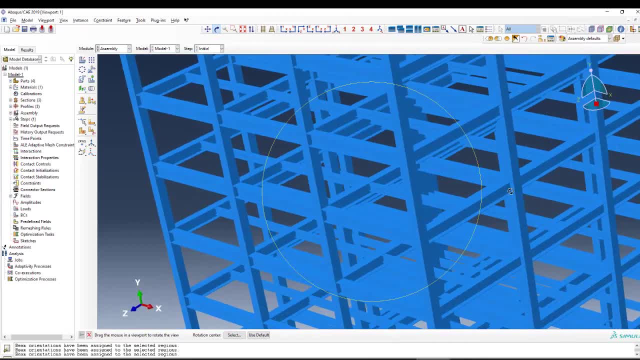 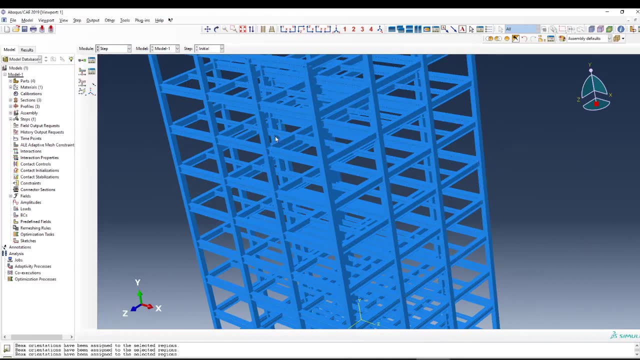 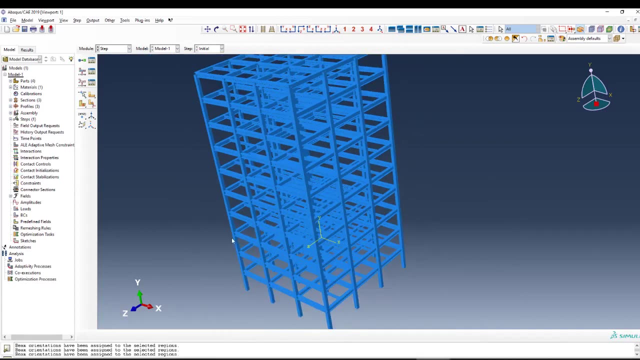 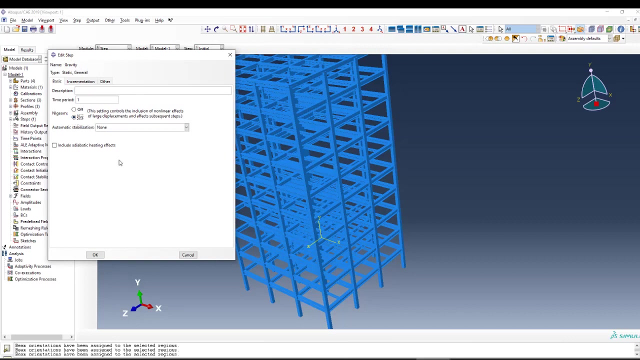 orientation and we see here, and this one also, all the beam is correct. next we're going to step. the first step is the gravity loads of this structure and we should define a gravity that can be static and we can turn on the NAMM. geometrical non-linearity and other parameters can be default. I like to use this called adaptive. 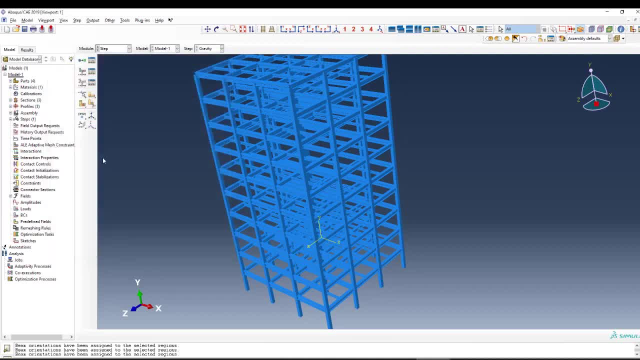 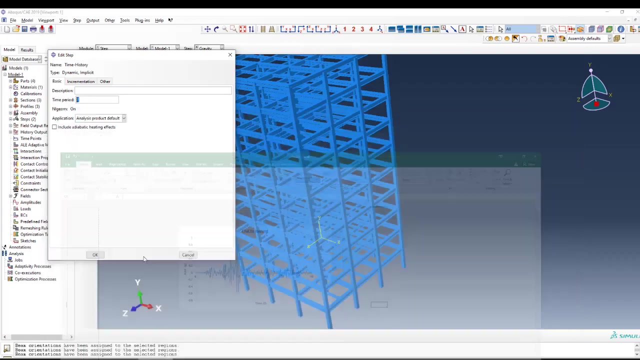 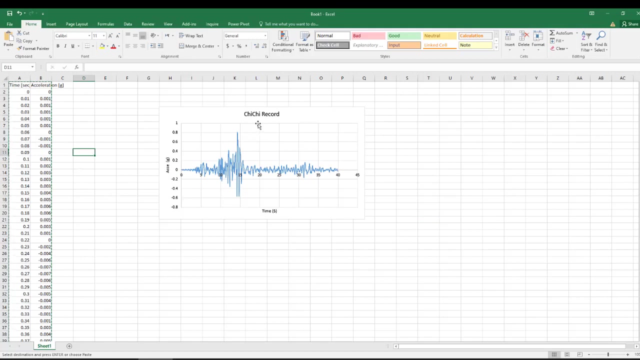 stabilization that can prevent from some of the errors. so the next setup is called time history and that can be dynamic. also, we can use implicit and explicit. so I interested to use implicit. the total time period is. here is a record I have brought from the. this is Gigi's record and I 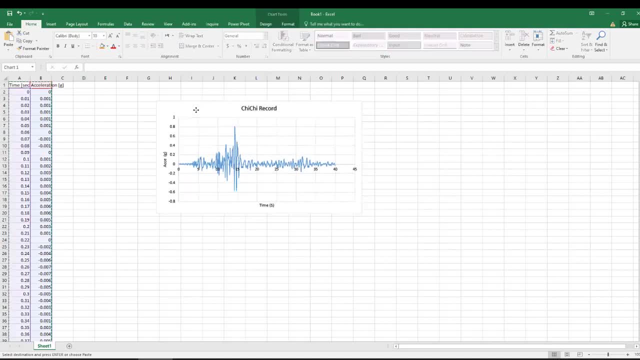 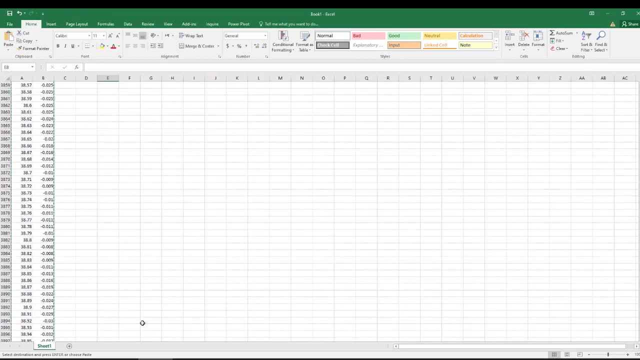 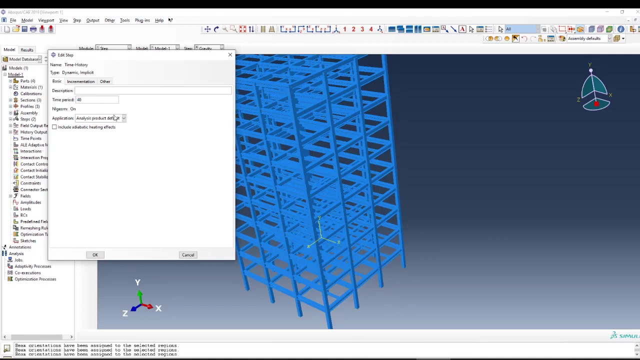 will show you how we can get this record or had a sort of records. the maximum time period is 40 seconds. now this is 40 second and I'm going to give days for these seconds. so using about ten thousand increment- actually here is four thousand and increased 10,000. 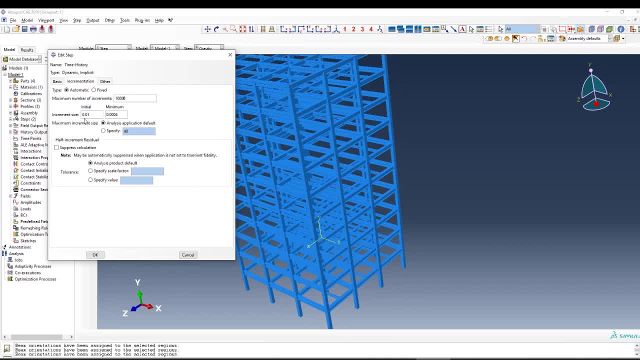 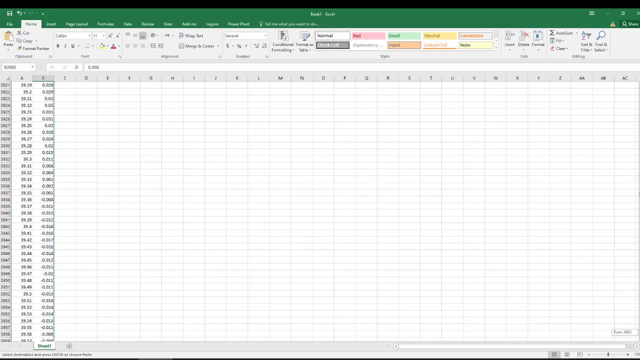 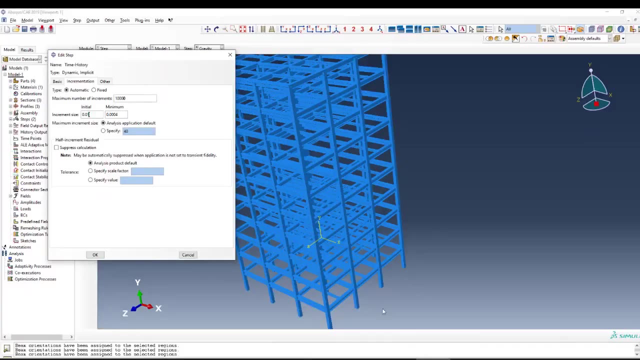 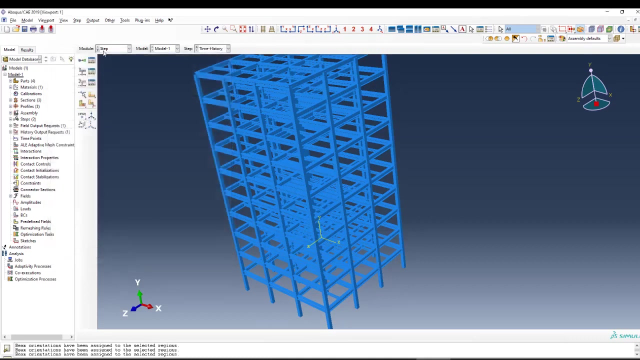 And the initial is 0.1, which is close to this time period- 0.01 second. And this is 0.01 second And the minimum should be something smaller, which is required to lower numbers. That can prevent also from some errors: 1E-15.. So other parameter is OK. So now we know it's OK And next is going to the load part. We don't need interaction or other things Going to quickly go into the load part. 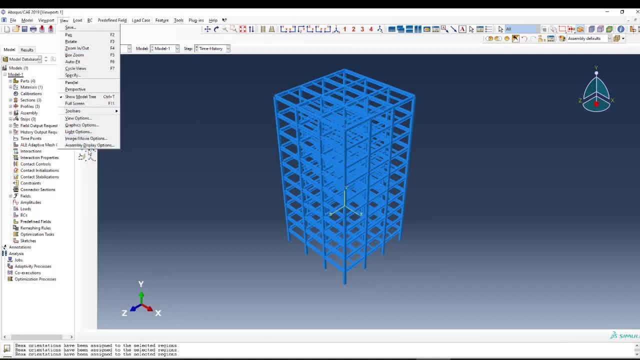 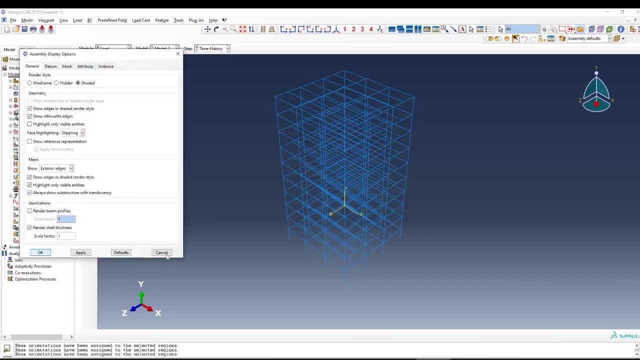 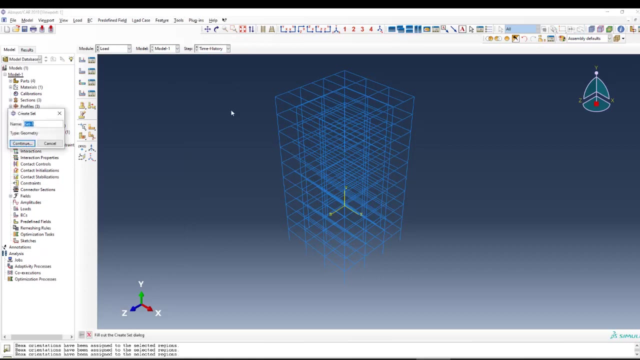 I'm going to turn on the load part, I'm going to turn off the assembly rendering Because we want to create a. OK, Here is a seat. I'm going to create a seat that's called the base nodes- Base nodes, And I'm going to select all those base nodes. 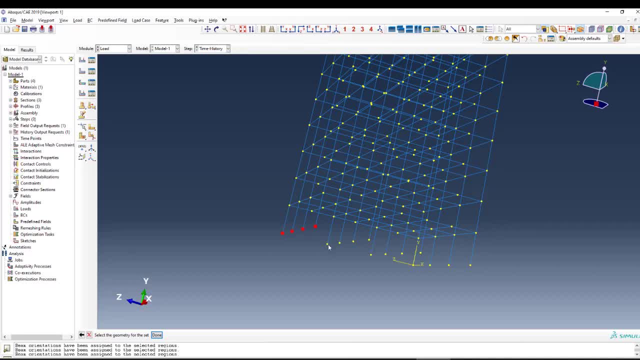 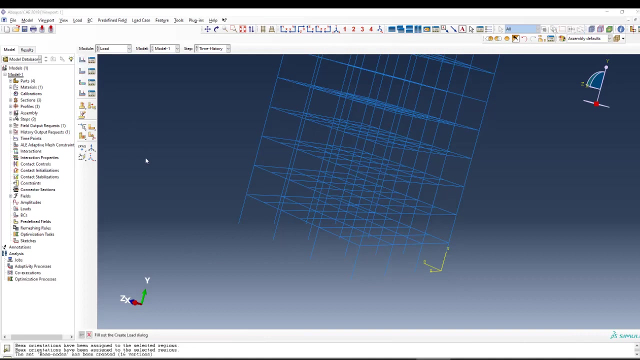 Boundary conditions. So here is one more. Now I can check. I should select all boundary conditions. So this is done. And next is going to apply gravity load, So I can call gravity load. The gravity load is something in a gravity step And here is gravity load, So I can select. So this is the if I give. we're using millimeters, So I should change the G to millimeters. 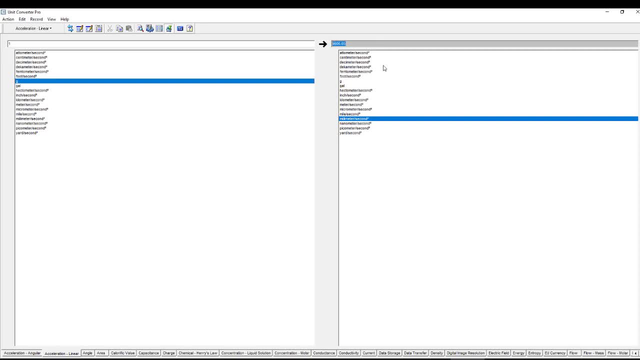 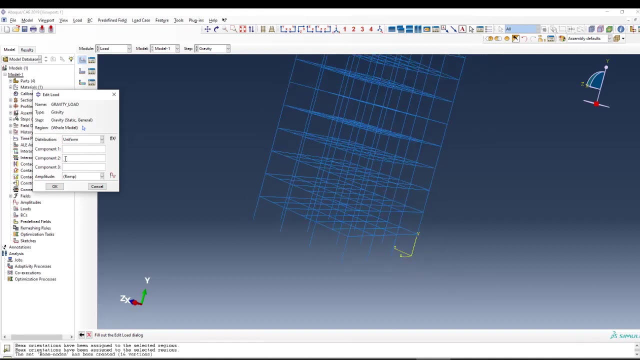 So 1G is about 9008.. This is millimeters per square second. So I'm going to paste this in direction. This is Y direction, with a negative, It's a negative And it's OK. So now it's gravity load. 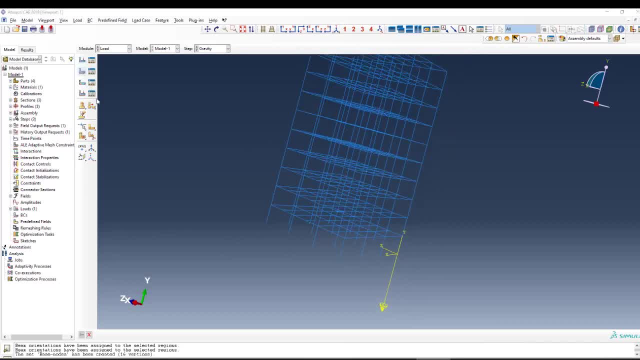 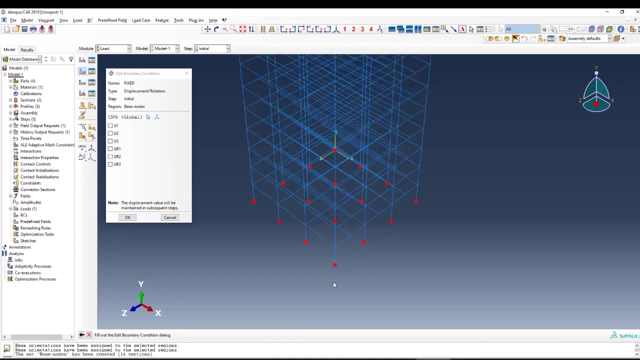 And the second is I want to give a boundary condition That's called Base of fixed. It should be an initial And I used displacement. Use that seed. Yeah, OK, I want to apply The The Ground motion in the base. 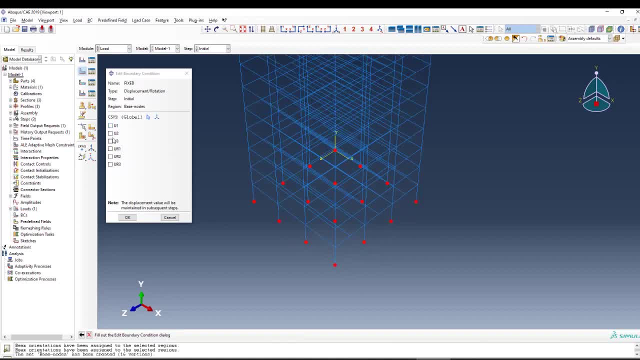 So I should Unchecked that direction During the earthquake. Other Can be Restrained, But except that X We assume to apply in the north of the structure. So this is You, is unchecked And the next is here. 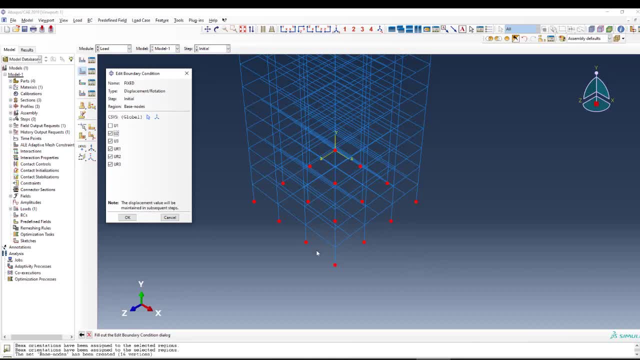 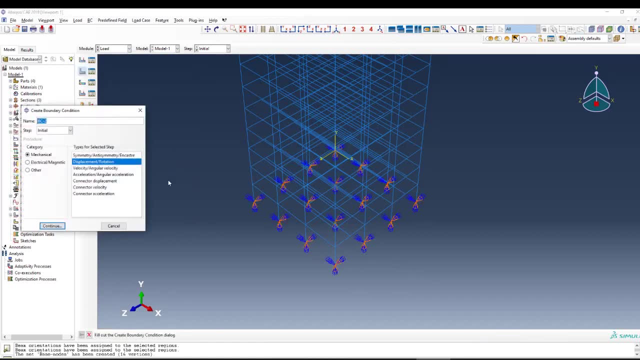 We want to apply The cold Time History. Time History Should be in a time history Should be in a time history. And the next is Here. We want to apply The cold Time History Time. 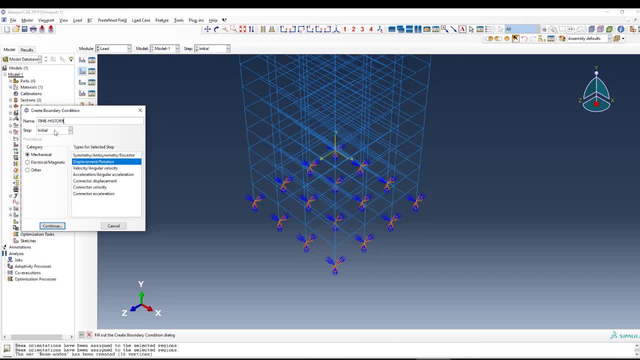 History Should be in a Time History Should be in a Time History. And using Uh Uh, We have. We can apply Velocity, Displacement And also Acceleration. I want to apply Acceleration. 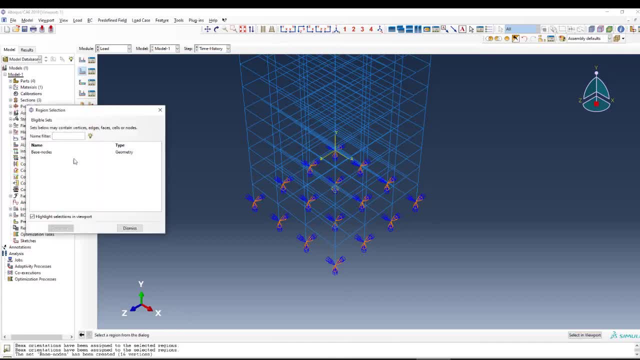 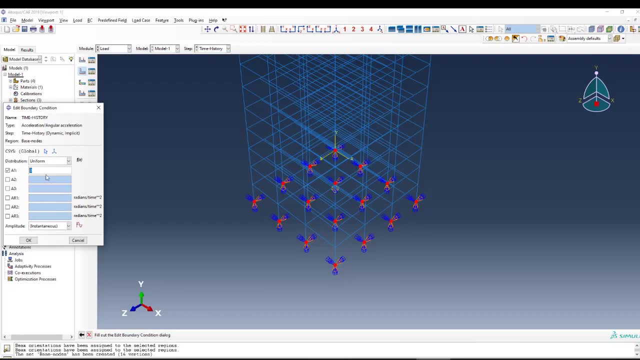 And it is called Acceleration, And Using The same Nude In a One Uh, This is G, Uh, We Have This data. Is G With The same Uh? Then We can. 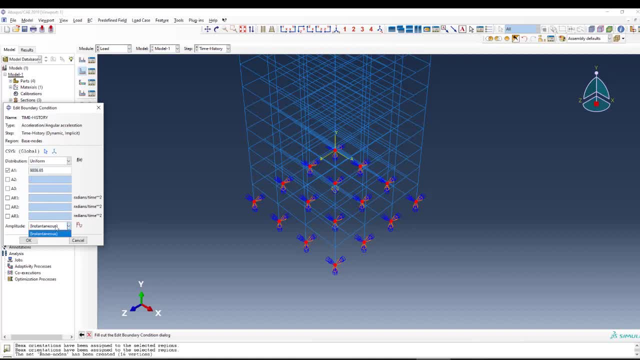 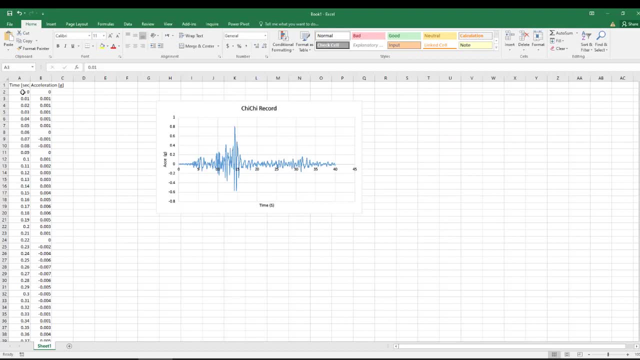 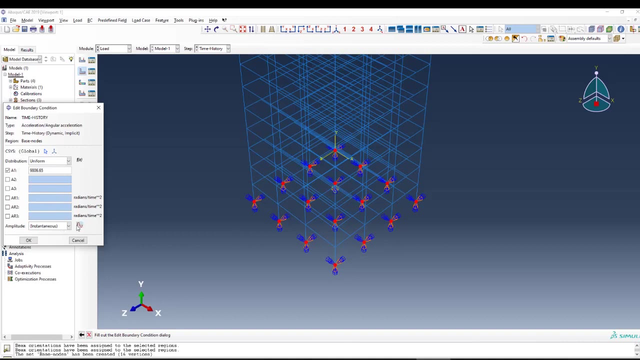 Give That Uh, Uh, Uh Parameters Here, So Here Should Be Applied. Uh, Um, We Should Apply These Uh Time Histories, So I Can Select. 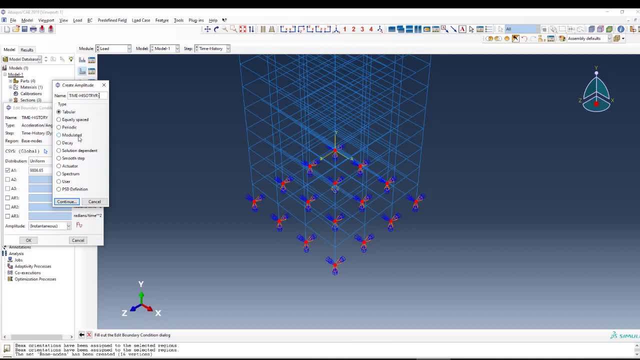 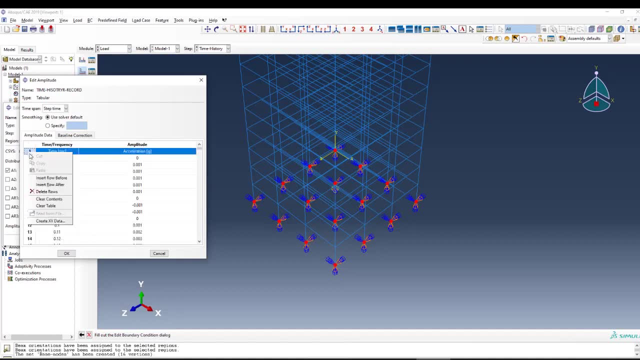 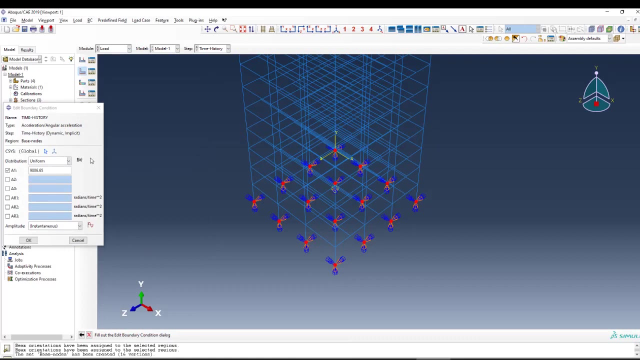 Uh, Record Record. Uh, Now I Can Paste, Here Is Paste. So I'm Gonna Delete These First Rules And Now It's Began Zero To. 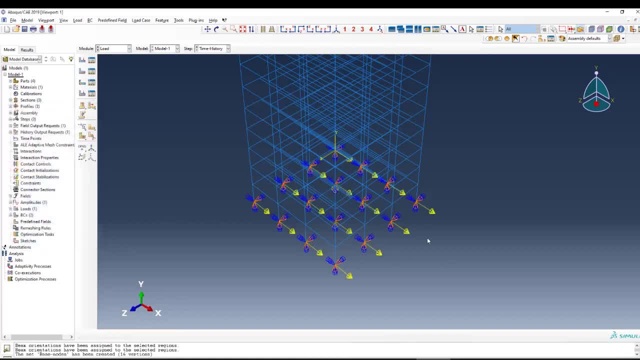 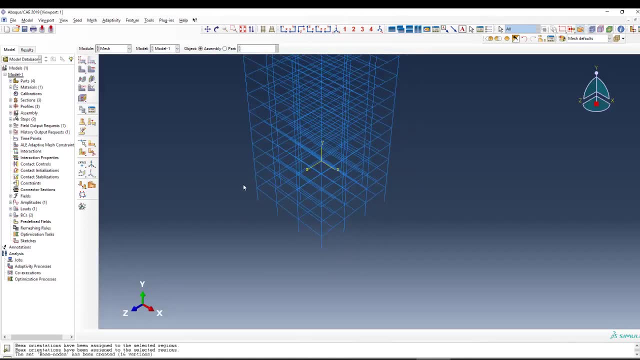 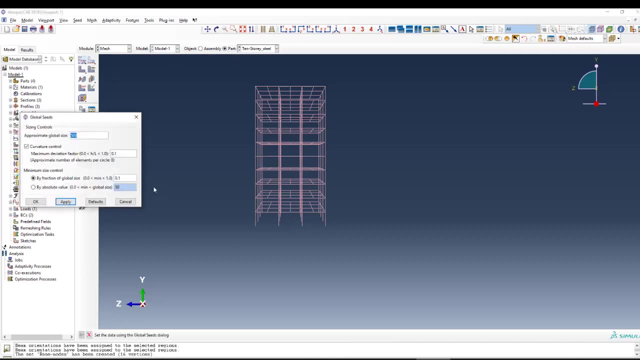 Zero And It's To Forty Second. Uh, Everything Is Done And The Next Day Is Going To Apply A Mesh. Uh, It Should Apply The. 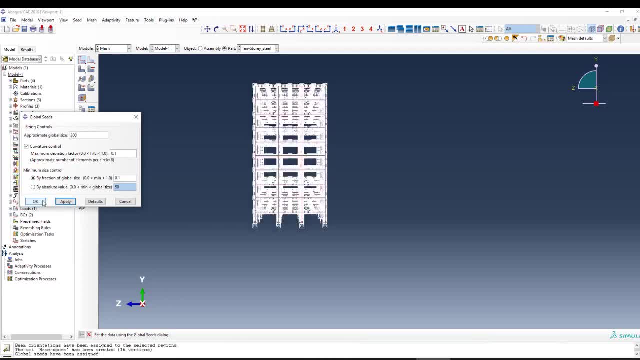 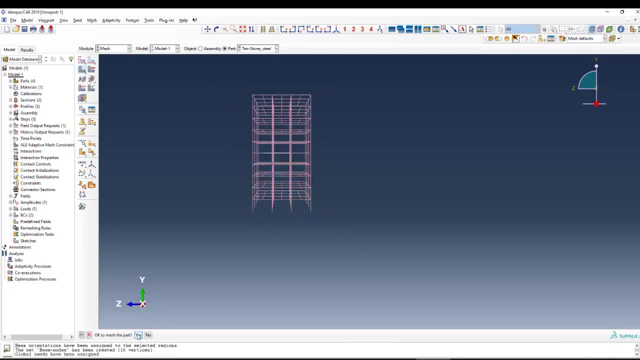 Boundary Limit In The Pots? Uh, We Can Use A Mesh To Determine The Type Of Elements. If You Don't Now We Can Select And. 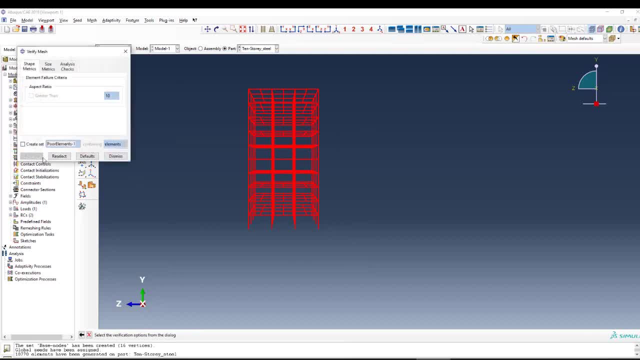 Here Is Already Selected B. This Is One Of The Issue. Sometime It Will Be. Here Is Let's See. Here Is An Analysis We Have. 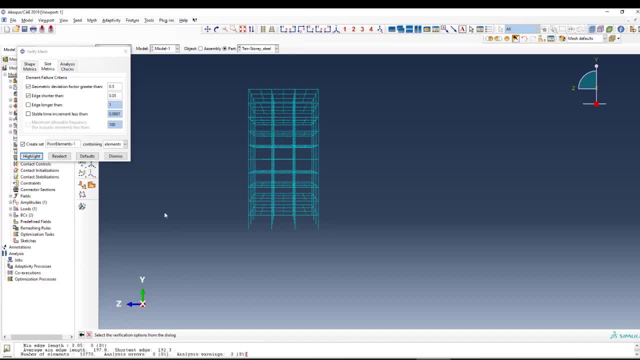 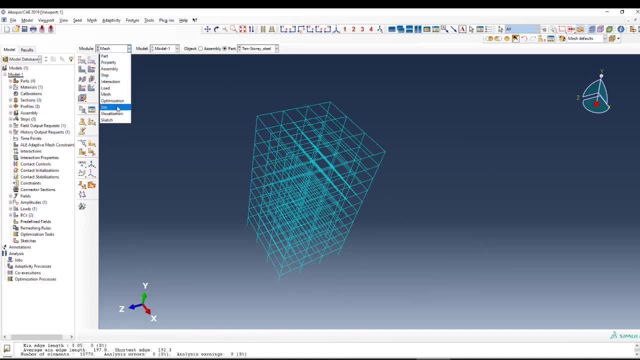 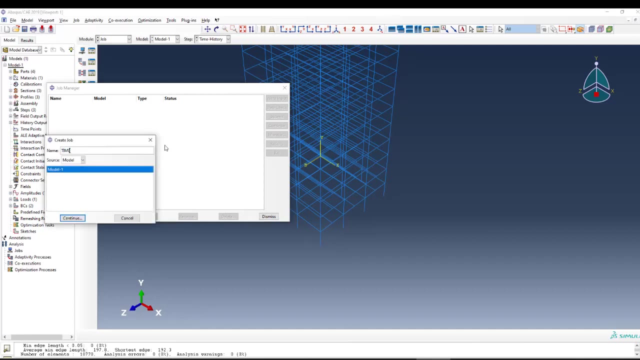 This Type, This Amounts Of Elements, And We Have Done. This Is Zero And Warning Is Also Zero. Time History Response. Sometimes We Call Time. 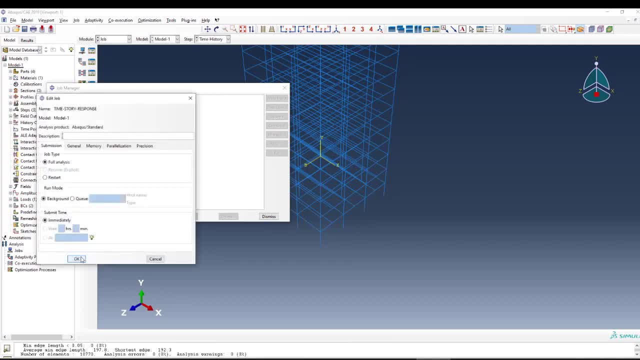 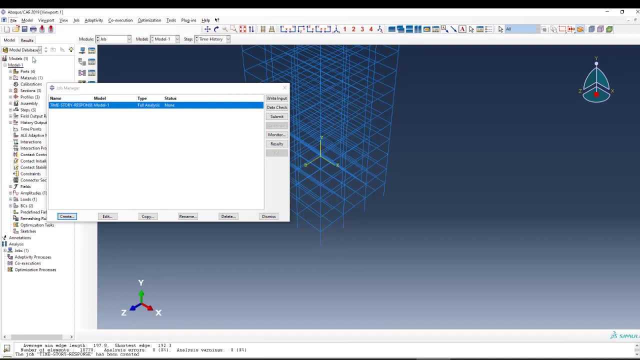 History Analysis, Also Time History Response. So Using The Default Parameters And Submit. But Before Submit We Are Going To Save Our Analysis. Okay, Now I'm. 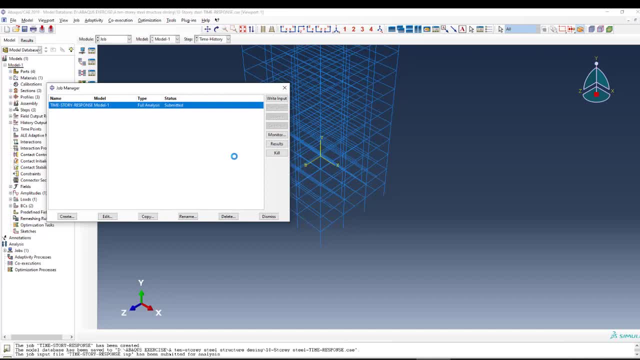 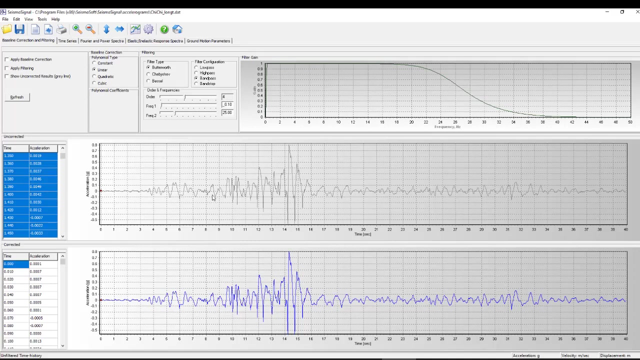 Going To Submit For The Analysis. Here We Can Check That Our Analysis Is Completed Successfully. We Can Go To Do One Thing Here I Have. 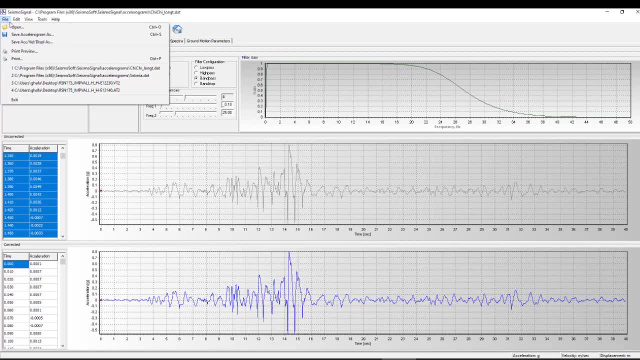 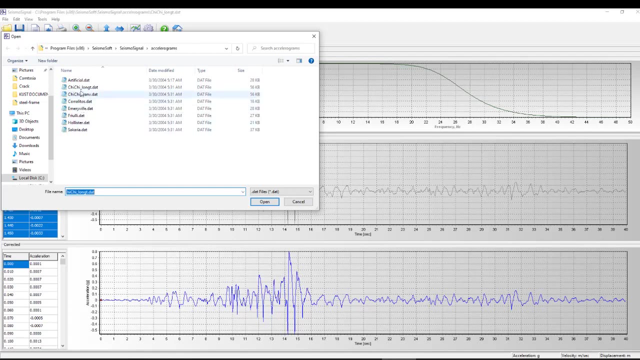 A System, Signal Software, Which Is Very Effective. So If I Need To Have This Software You Can Open. Here Is Some Axial Grams Already. 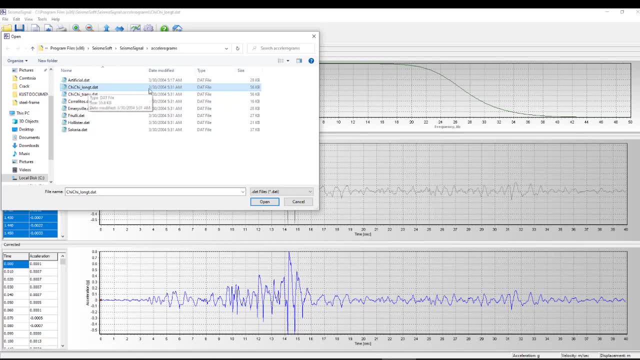 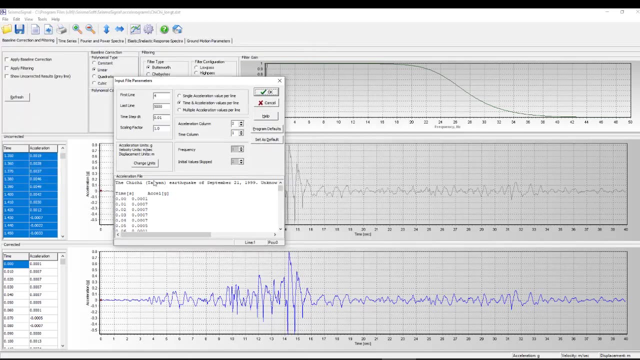 Saved In This Software Directories. You Can Select Any Of This You Want. This Is A Long And We Can See Here Is Called Time. 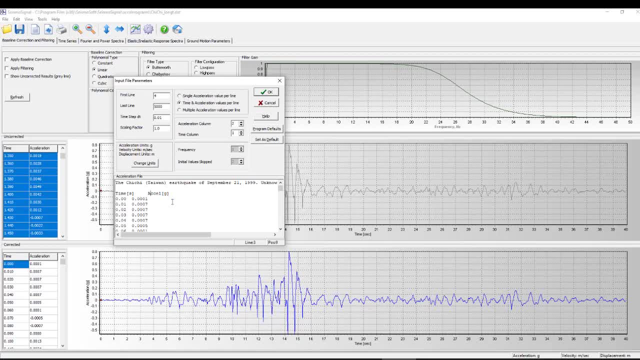 And Is Acceleration? Here Is The Option You Can Select. It's One, Single, You Can Say Single Acceleration. If It's Multiple, Then Say This: 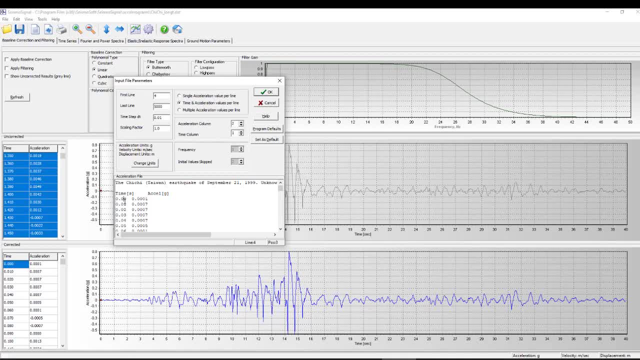 Is. Column Two Is Acceleration, And Column One Is That The Time Period Is Already Written. Here. It Is Also Giving The First The Difference. 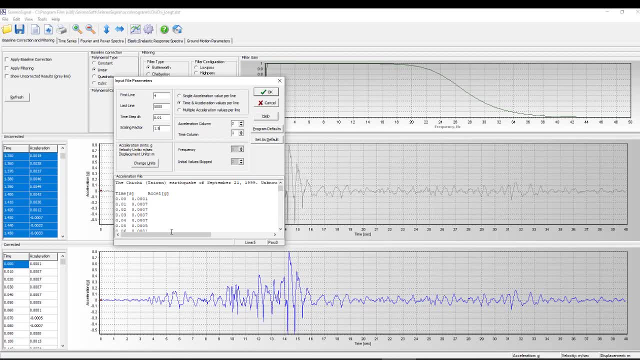 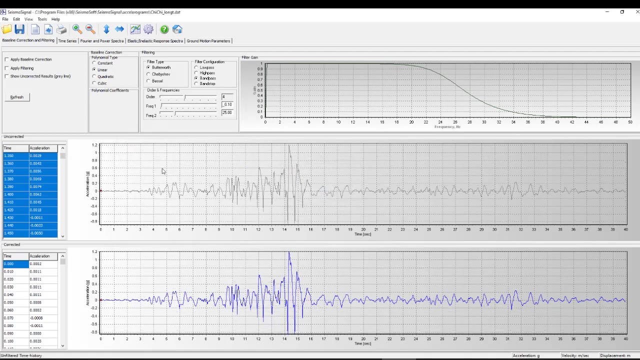 Between Scale 50% Of This Acceleration And Then Apply To The Structure. Well, What Structure Response Now We Can Called End Of The Reach 4500.. 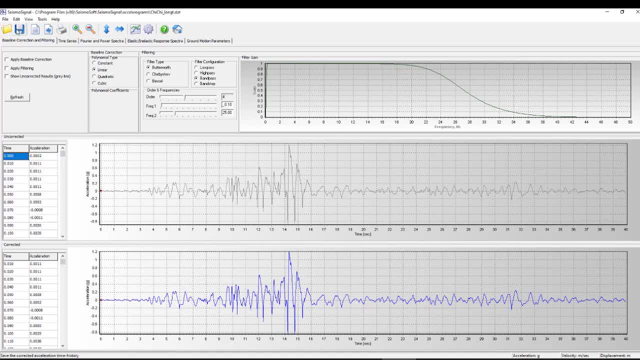 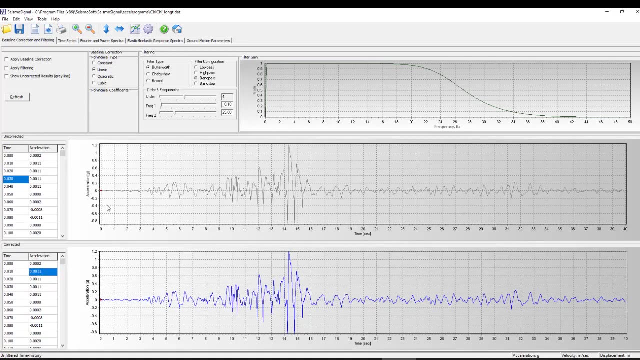 So This Is The Record. It Is Acceleration, Or We Want To Get The This Acceleration Fix It. You Want To Use This One, Or 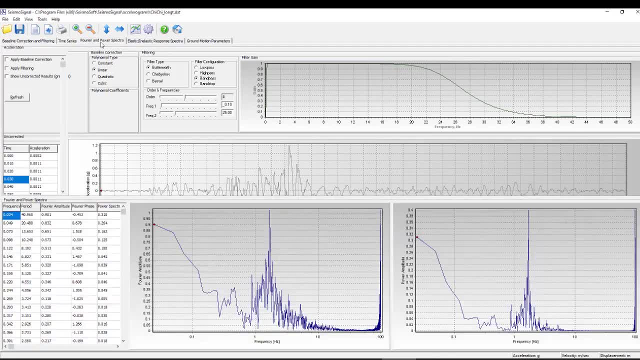 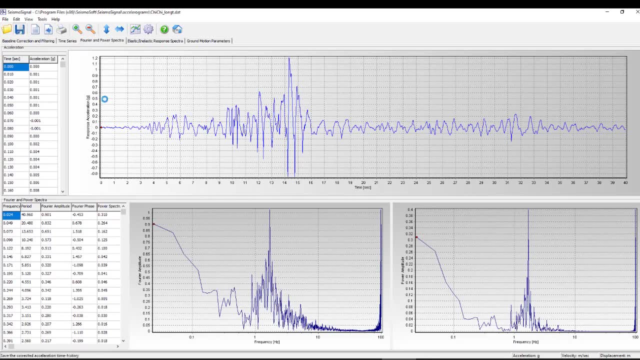 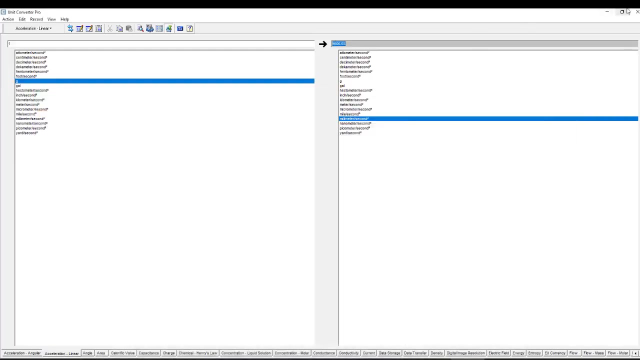 This One Correct Some Parameter We Can Correct. Or And Also To A Text File Here Is Called Time History Text. Yeah, We Already Have. Then 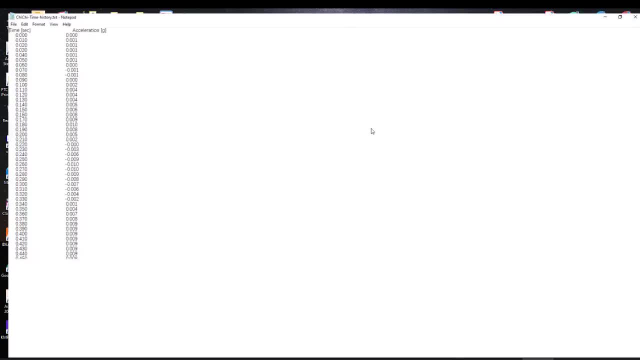 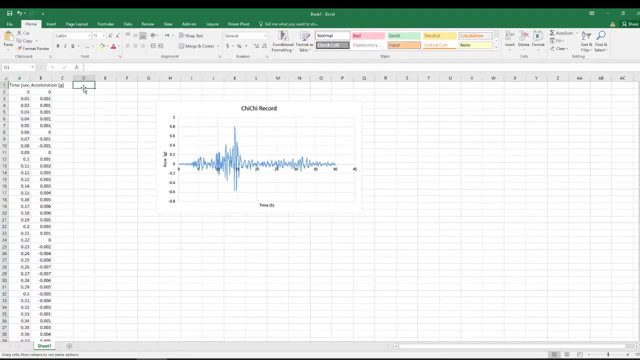 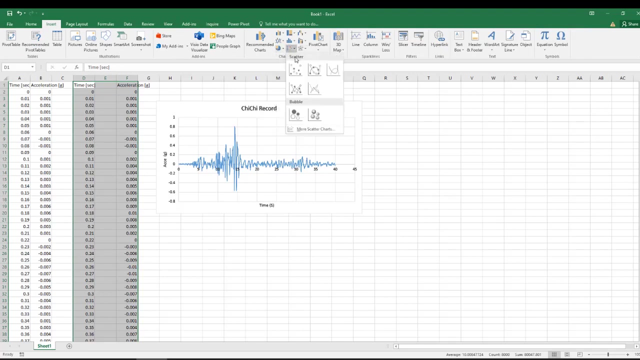 I Can Go To The My, My Desktop. I Have Recorded In Desktop. Here Is So This Was One And This Is One Point Five. So 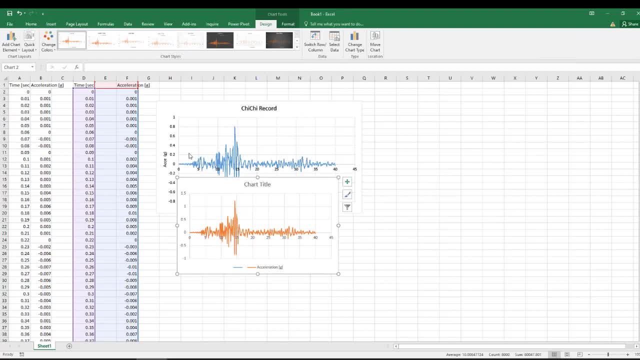 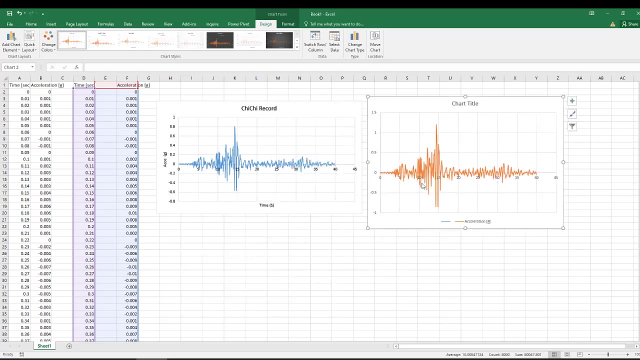 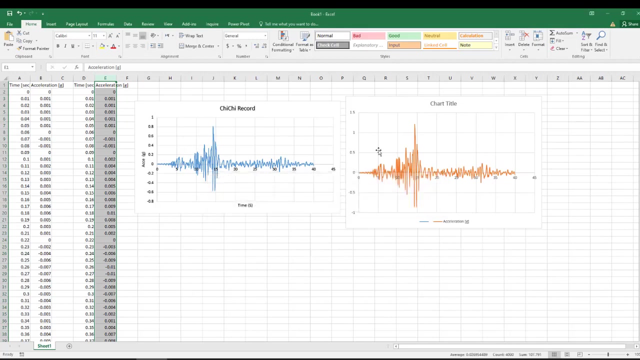 I'm Going To Select And Insert, Insert Curve. This Is The Curve, This Is, You See This, One, One And Select. We Can, I Can. 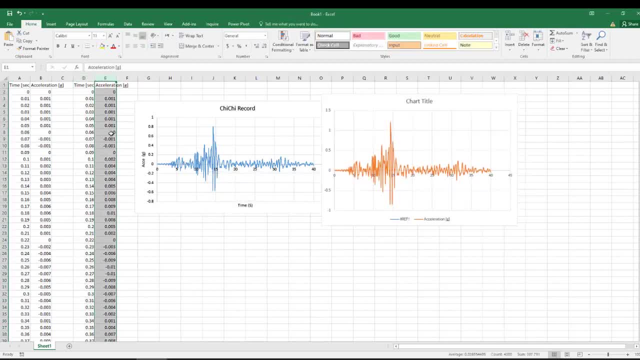 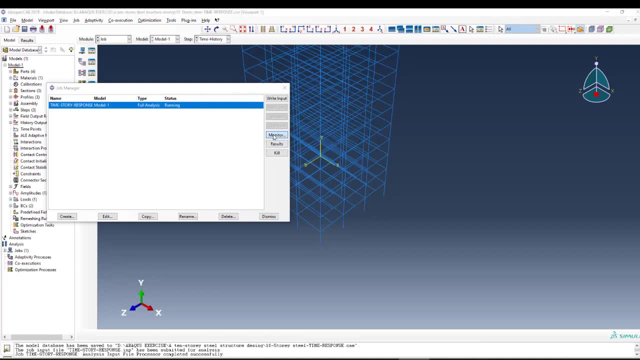 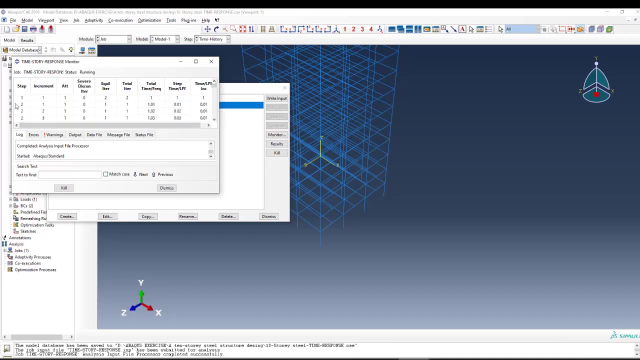 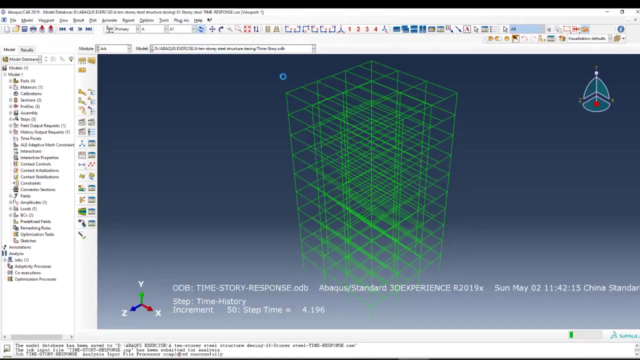 Remove This Column And Then I Can Select All This Column, Like I Update, To Perform Time History Analysis. Now We Can Check. This Is The. 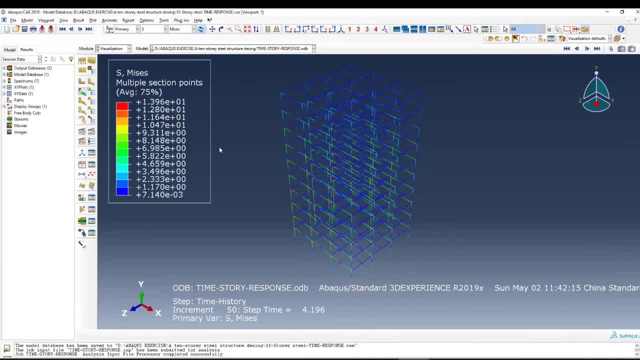 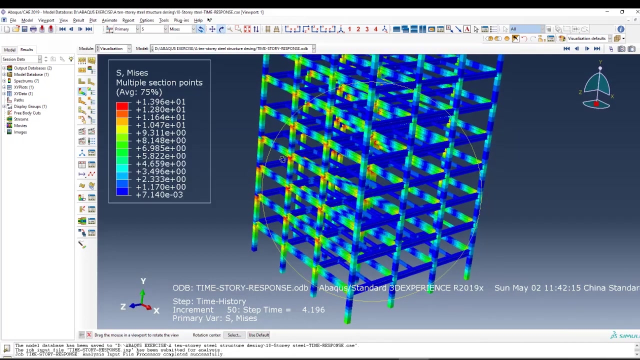 Result. We Are, This Is The One Message Response And We Can Go To The View Display And Turn, Check The Rendering And We Can See. 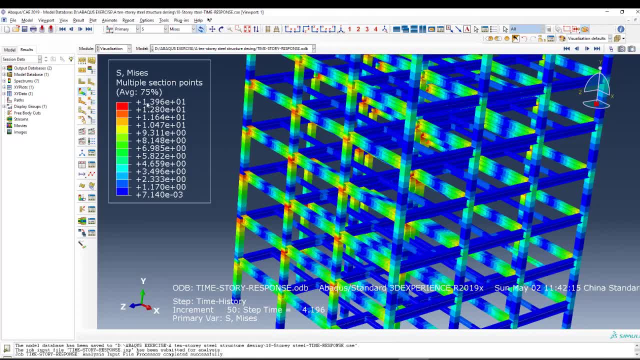 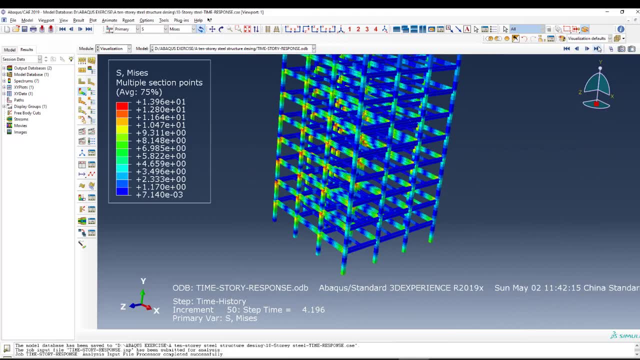 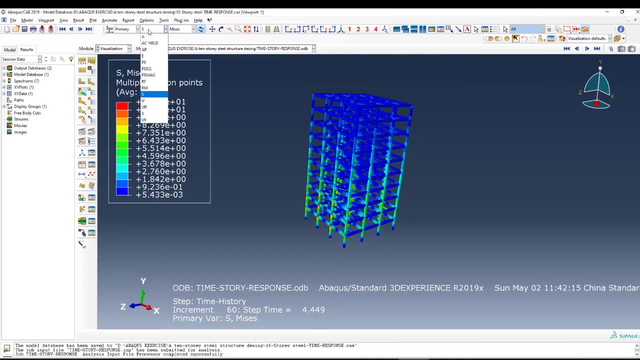 How This Will Damage, But This Damage Is Less Than The Allowable Damage Yield Stress. So Still, The Structure Is Safe And We Can Continue. 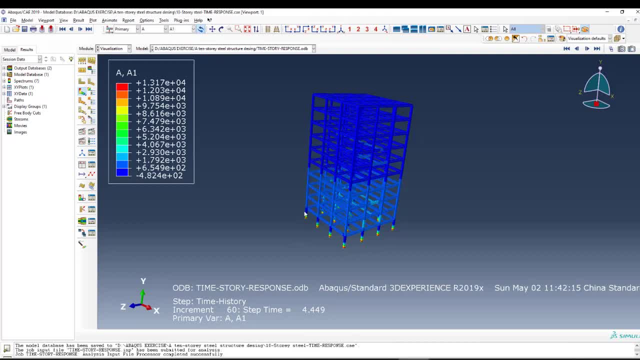 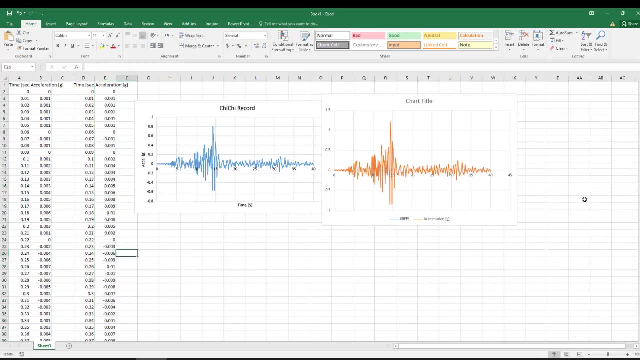 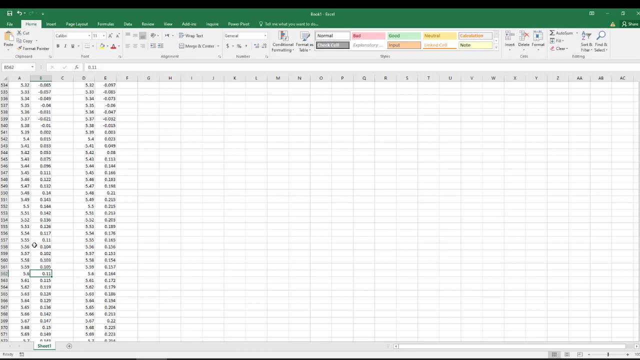 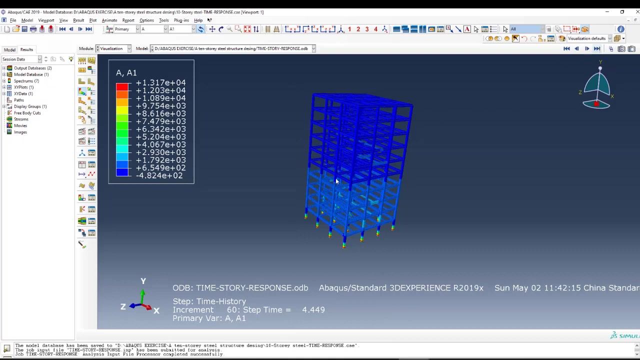 To See, And Also because the first about four second, the four second is not too much, not too much large formation here. this is five, very small and with which it is done or it's finished, at least in the maximum in the here. yeah, now it's going to the top of. 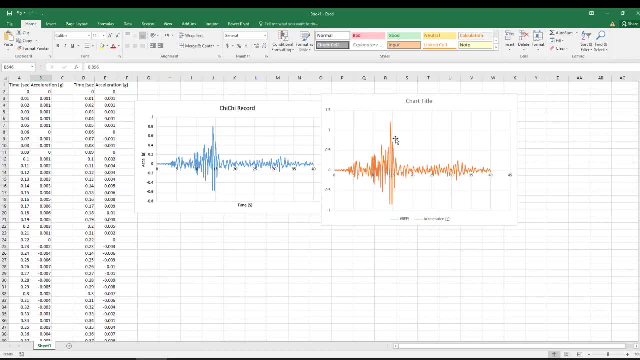 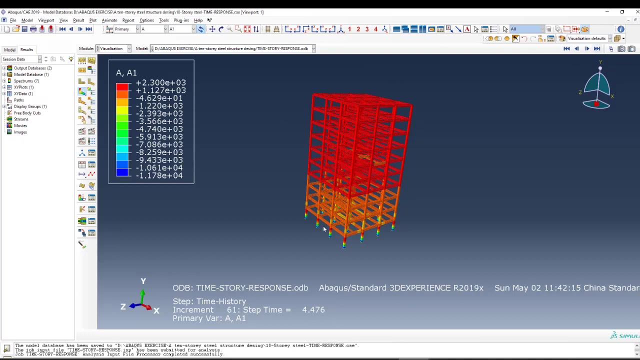 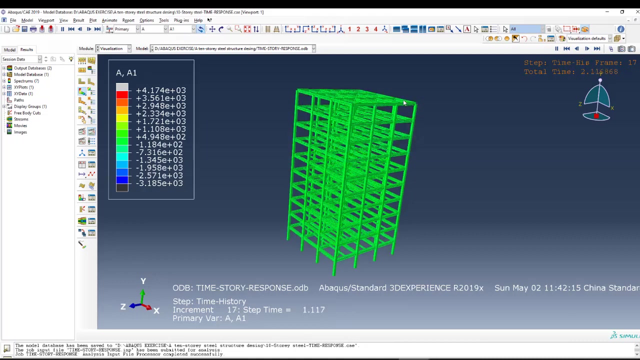 that when it comes to this region about 10 and 15, so the structure top roof acceleration will increase like this. so now we can see the maximum is going to the top. here we can use the animation and see: here is some. yeah, this is animation is going to show you how they. 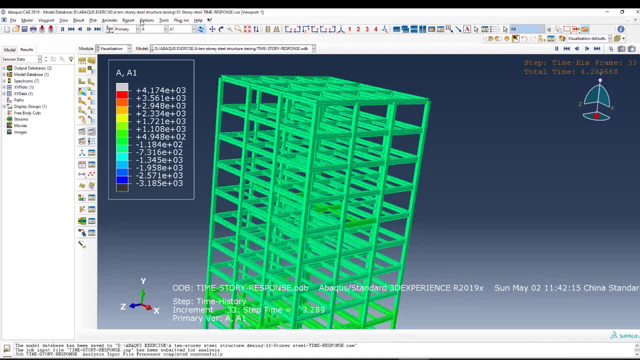 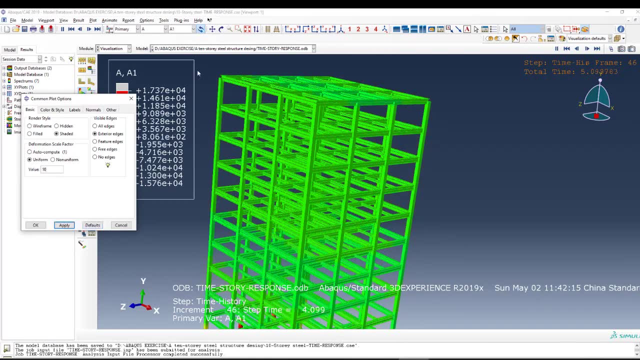 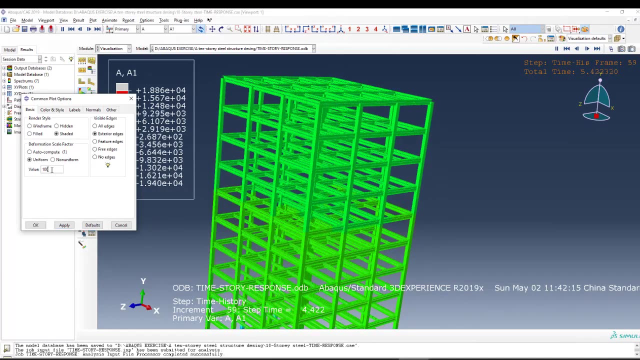 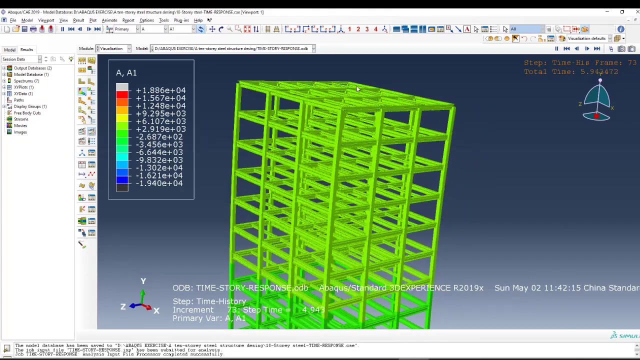 spread because, yeah, so that I can extend to 10 and you can quite quietly see the acceleration in the top or bottom. yeah, now you see and see. Let's say, if I increase 200, we can see, if I increase 200, we can see. Yeah, this is acceleration. 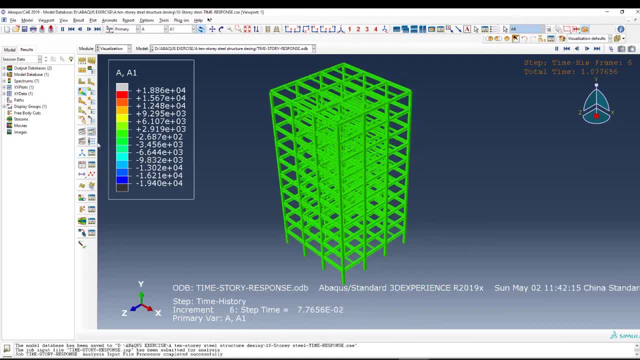 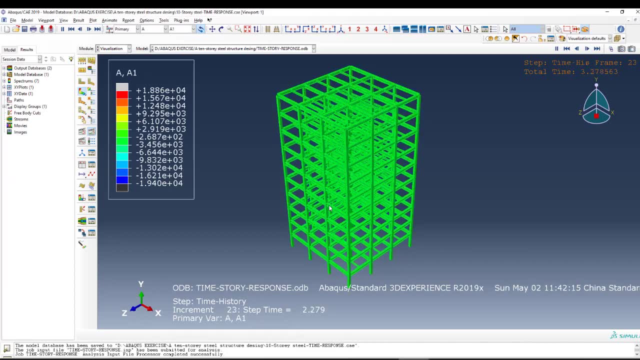 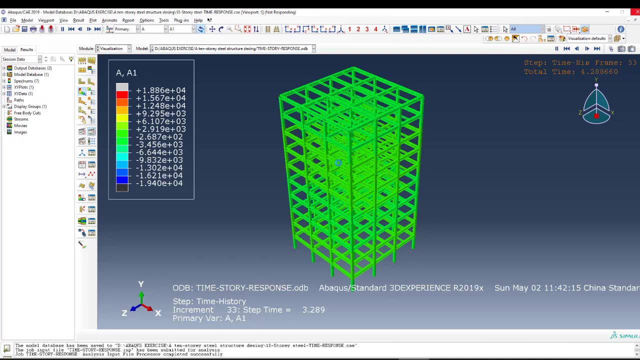 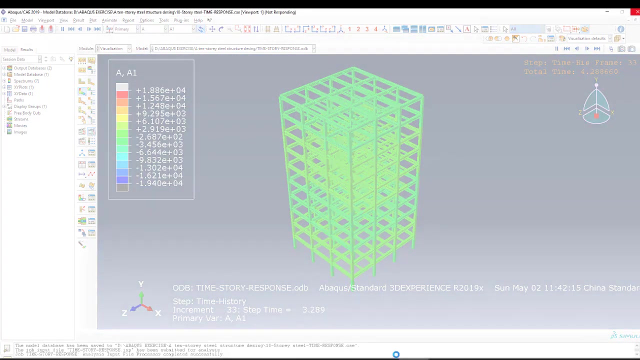 Now let's see. this is the acceleration same Yeah衝. This is deliverable acceleration. so it's because there's a lot of nodes and elements. so the computer making slow, I will. I will keep it to finish after the finished. now I want to post a video after finish we can see. 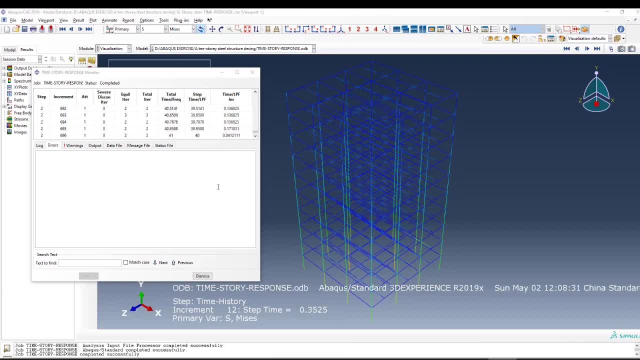 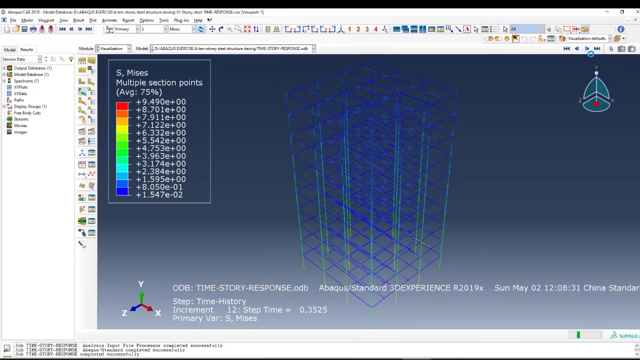 some reason now the analysis completed. here is the logo which is we submitted on 12, 12 o'clock and now it's completed about almost 40 minutes so we can go to the see some results. here is the stress string curve, three string deformation and we can. this is the strain stress deformation. we can take who to be failed. 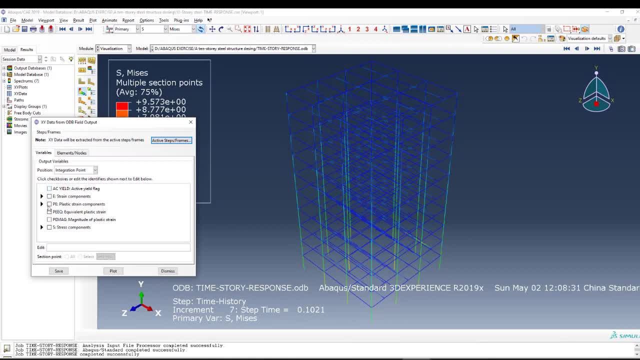 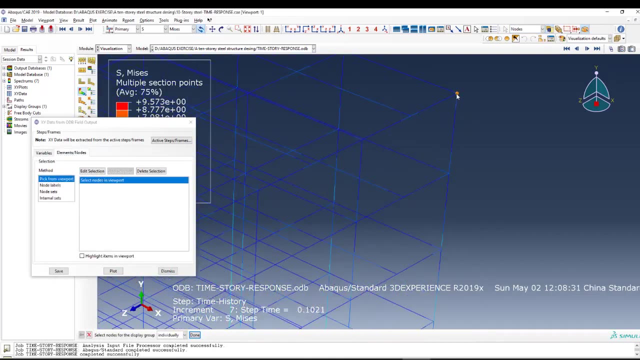 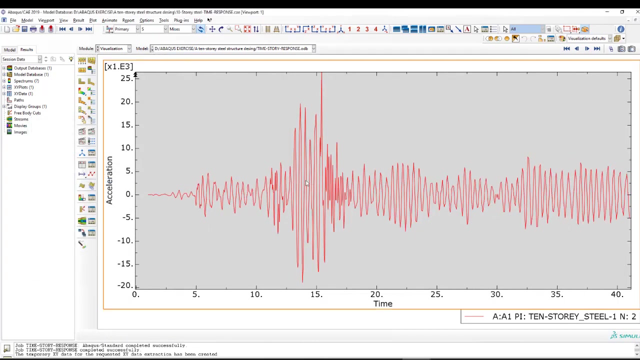 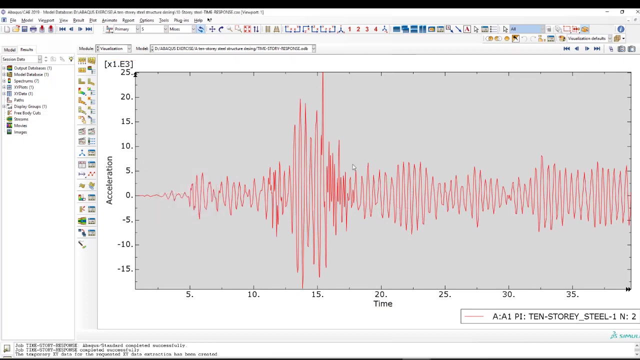 out but- and we can take who to be failed out, but from unique no notes we can select. this is acceleration in u1. select a point. I'm going to select this point and plot. this is the response of the structure from top on the top of the roof and also. 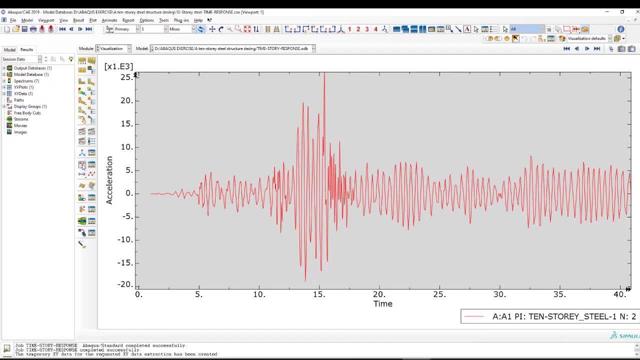 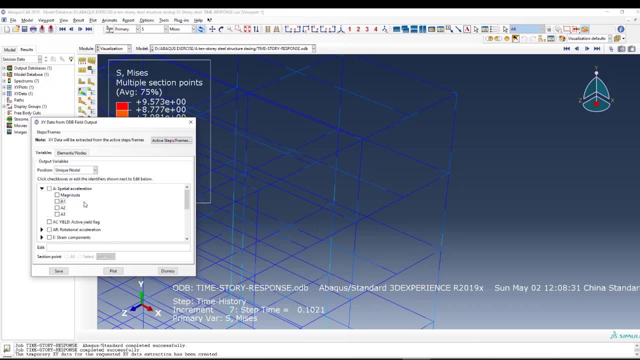 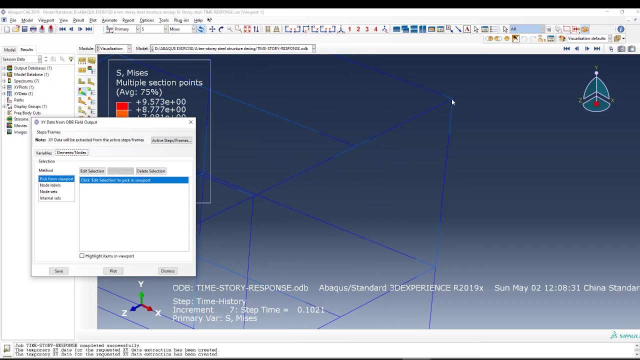 we can plot. we can plot the vibration velocities going to here and select output. the same here is turn off, here is called velocity and this is a special velocity in u1. at least should one node select when we set the speed, for example for a forward retreated Benz. 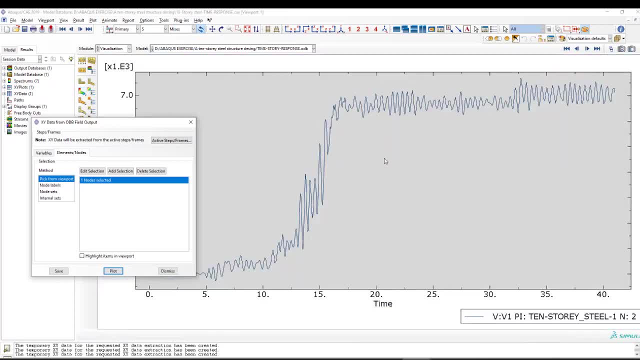 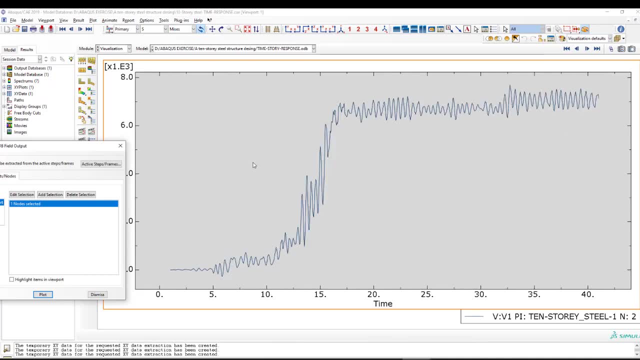 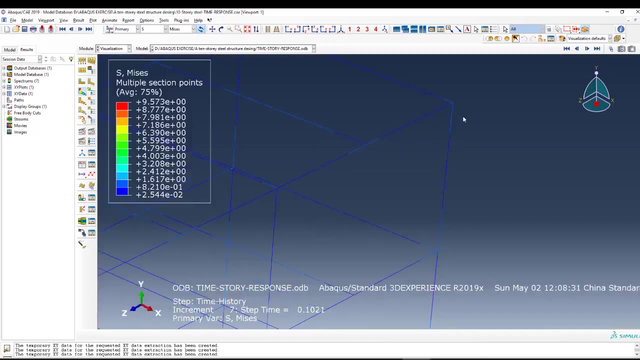 we can plot. the battery will be in my. so e is equal to that and a assigned point here is the green and minus, so it isut. ti is equal to zero, so is the speed in a to ground motion. so what's the response of the structure? so most of time the